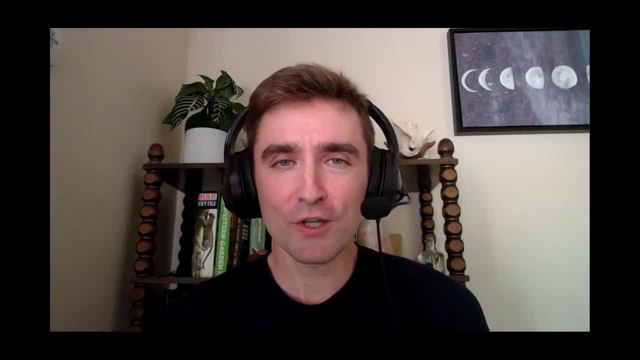 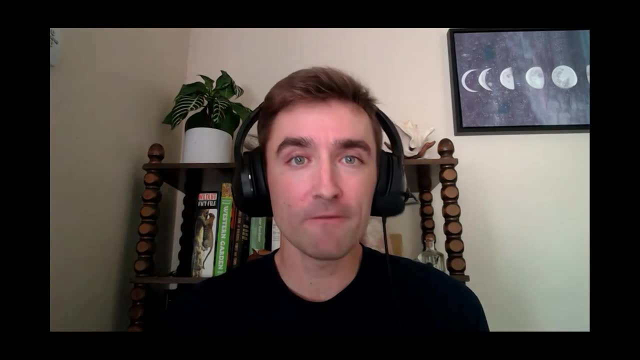 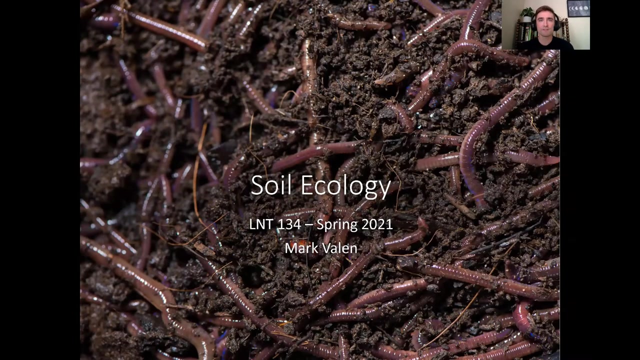 All right, let's talk about soil ecology, And really what we're talking about is life in the soil and how the living things in the soil interact and support plant growth. This talk used to be called soil biology, because really all it was was a running list of all the living 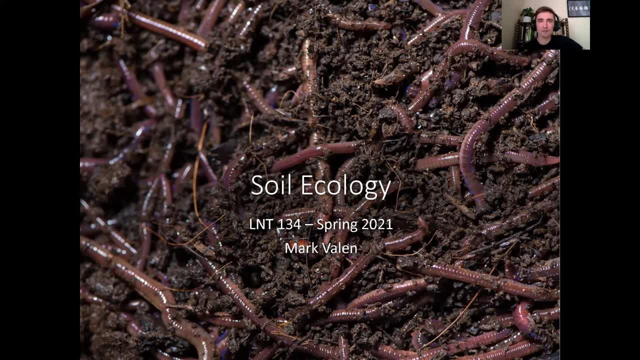 things in the soil, And that's how soil scientists used to think about the living things in the soil. Well, what are they? Let's classify them and let's describe them, and then let's move on. But now we think of it in terms of ecology, And what ecology is all about is 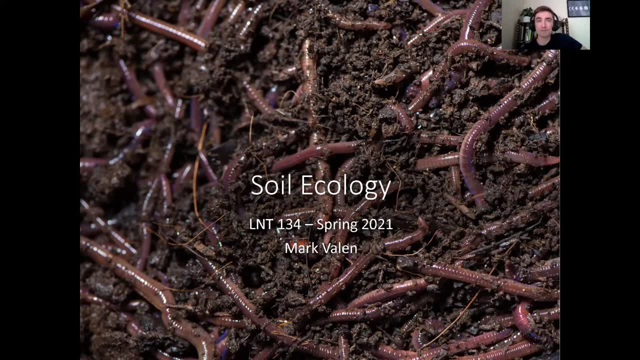 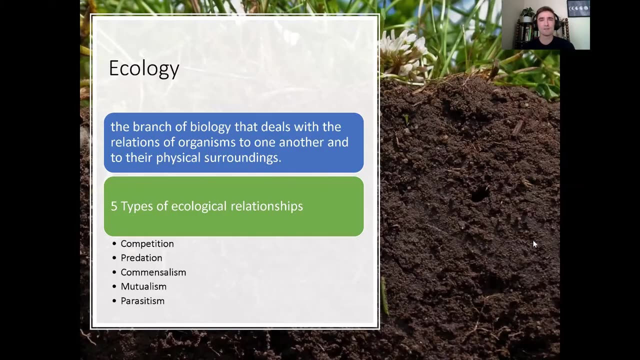 the function. So what are the organisms doing and how are they interacting and how does that interaction work With our plants? So we're going to get into a little bit of the biology and then the ecology as well. So here we go with a little definition of ecology. It is the branch of biology that deals 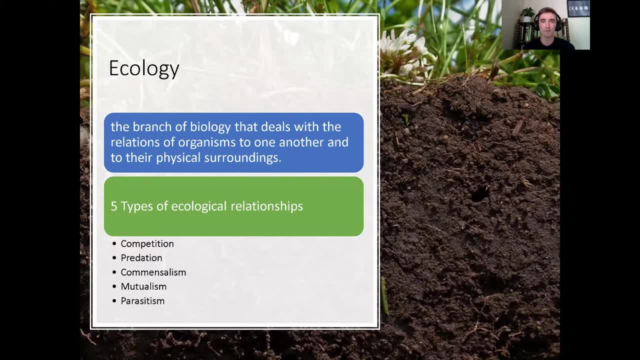 with the relations of organisms to one another and to their physical surroundings. So we have the biotic and the abiotic components of an ecosystem And there's a lot of interactions. There's a lot of, there's a lot of relationships Taking place between all the component pieces, And ecologists define five general types of. 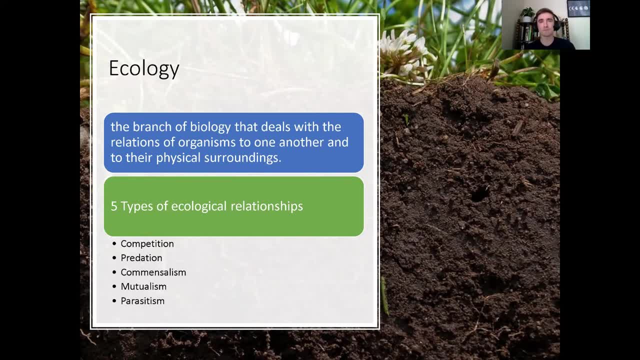 relationships or interactions that different organisms can have. They get a little bit more detailed than that, but this is a good generalization. So we have competition and we're familiar with competition, which is one organism eats all the food The other organism cannot eat. 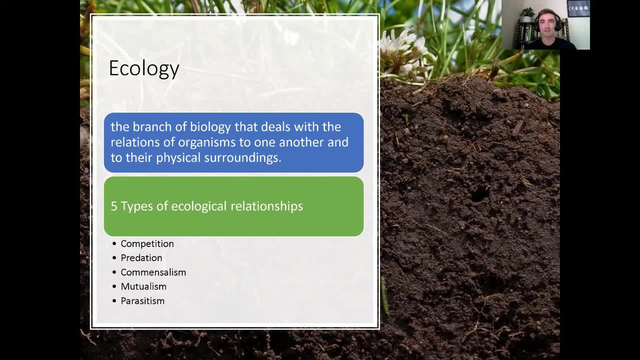 the food, And so therefore, we have two different species and they may compete for the same resources. Then we have predation, which means one animal eats the other animal, And in this case plants are included as well. So typically we have animals, organisms that eat plants. 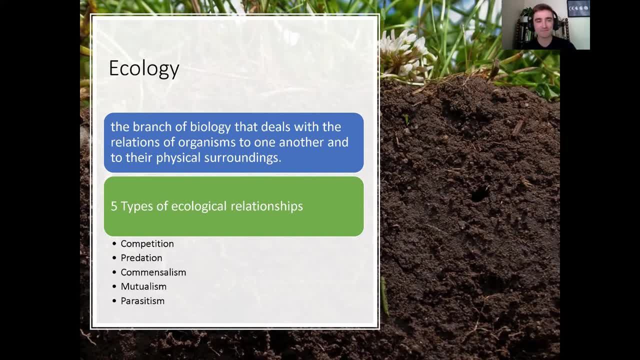 Although every now and then plants will eat animals too. And then we have commensalism, And that's where one organism benefits and the other has no benefit, neither positive nor negative. So it helps one, but it doesn't matter to the other. 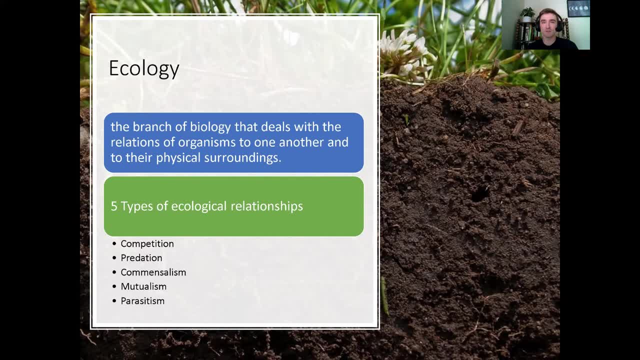 And a classic example of this in nature is like a shark, for instance. the shark has those little smaller fish swimming underneath, and the little smaller fish can take a bite of whatever the shark drops out of its mouth, And so it's good for the small fish. 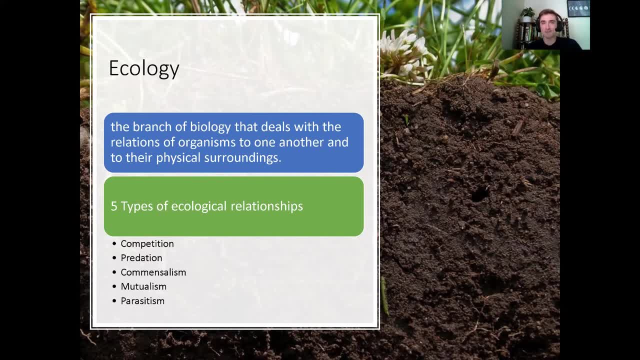 but the shark doesn't care if it has the little fish there or not. It doesn't help the shark but it doesn't hurt the shark. So that's called commensalism, when it helps one and it has no impact on the other. And then there's mutualism, which is where both organisms 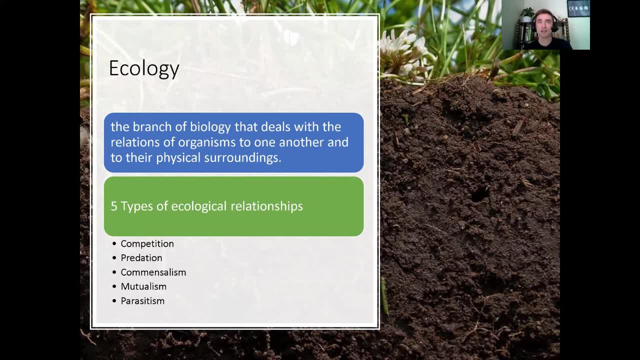 benefit. So this is your classic pollinator example, where an insect may visit a flower and get a food source from the flower, And then the flower- the plant- gets the benefit of pollination in return. So they're both getting something positive out of the experience. 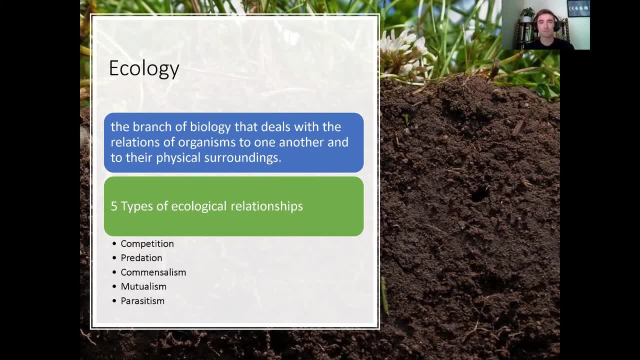 And then there's parasitism, which is where one organism benefits and the other organism is hurt. but it's different than predation, because with parasitism the one that's doing the hurting is trying to keep the other one alive and not kill it. So you're not eating it Usually. 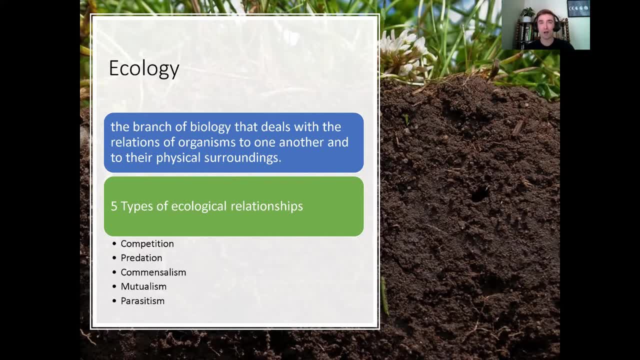 it involves reproduction, and wasps are very important parasites, but there are also disease-causing organisms that act as parasites internally for plants and animals, And there are some parasitic plants that are parasitic on other plants as well. So all kinds of interactions And 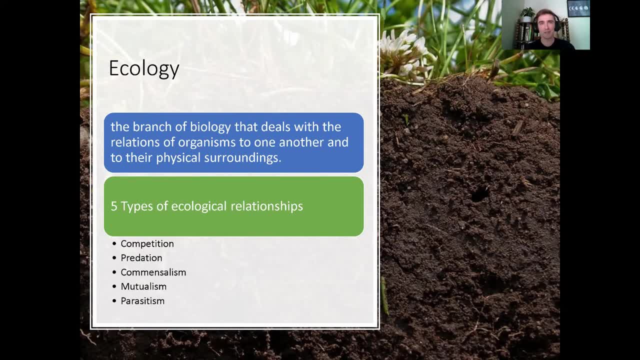 I mentioned just, between two individuals or two species, for instance, but these can be within a species, These can be two populations, They can be different species, They can be all together And they can actually be more than two. So imagine adding a third, fourth, fifth, 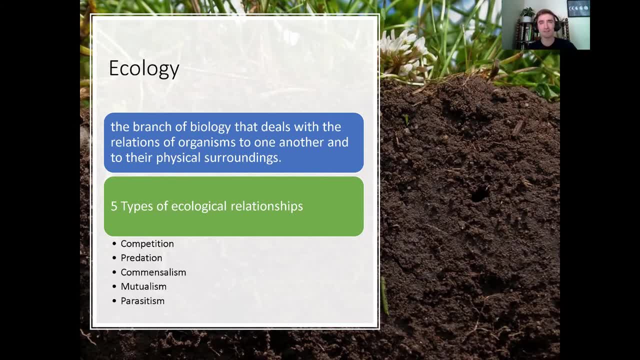 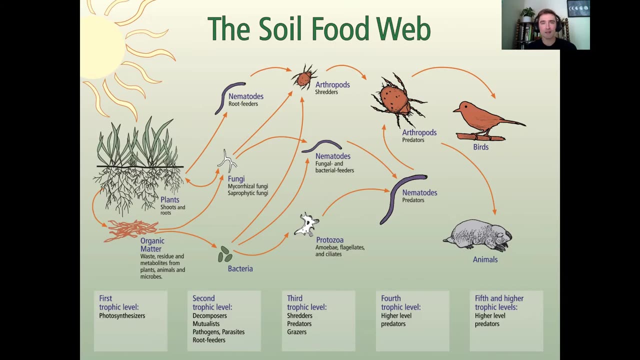 sixtieth species to this mix and they're all interacting in these unique ways. It gets quite complex, But this is the basis of ecology And we used to describe these relationships as a food chain, But now we recognize that a chain implies linear And that's not. 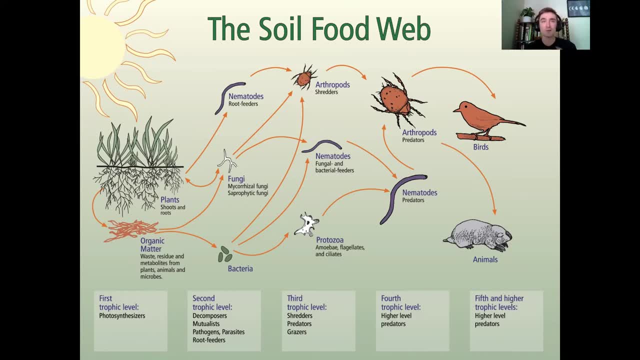 quite accurate. Sometimes things occupy different levels in the interactions And so instead we call it the food web. But still, with the food web, like with the food chain, we can find general categories And we call these categories trophic levels, referring to what it eats. And so in this, 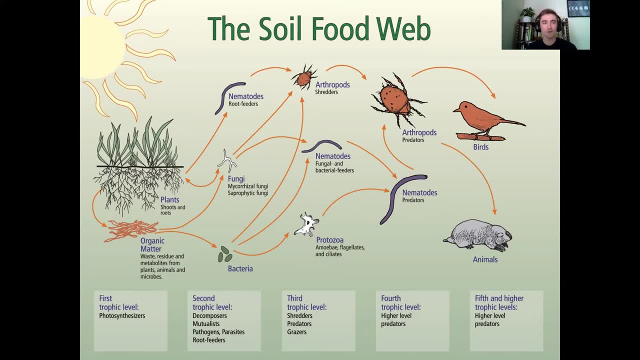 soil food web. the first food chain is the food chain, And this food chain is the food chain of The first trophic level are the plants, and the plants eat the sun. So, using photosynthesis and carbon dioxide, with the presence of water, the plants create the food with the energy of the sun. So that's the first level. Those are the photosynthesizers. That's the first trophic level. 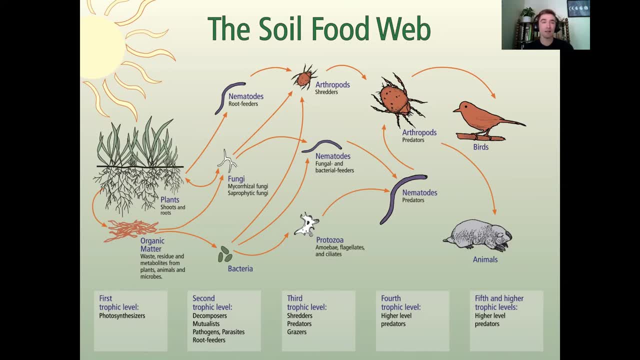 The second trophic level will be anything that eats the plants, And it could be living plants or it could be the dead plants, because plants will die and drop. leaves and roots are always dropping off, shedding and decomposing. So the second trophic level in the soil are the decomposers, the things that are actually breaking down, basically eating and pooping out. 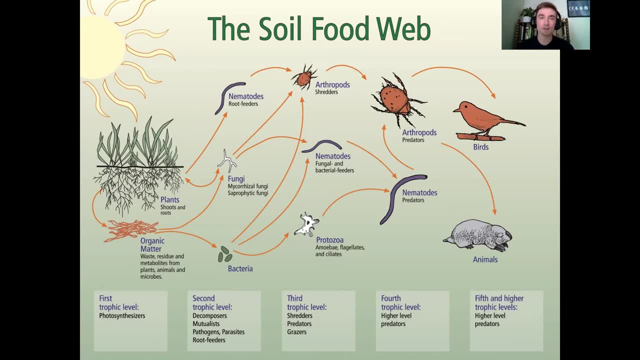 The plant material And obviously these are an important group. If you take a look at the plants and the organic matter, the arrows are going to point toward the organisms that consume them. So you can see bacteria and fungi will eat decomposing organic matter. Fungi will also go after living plants. 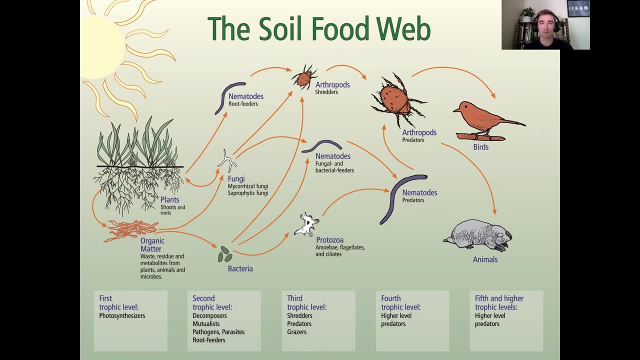 And then we have nematodes. These are little worms in the soil, microscopic worms Those can eat your roots as well. And so our second trophic level. the decomposers are the bacteria and the fungi, because they eat the dead organic matter. 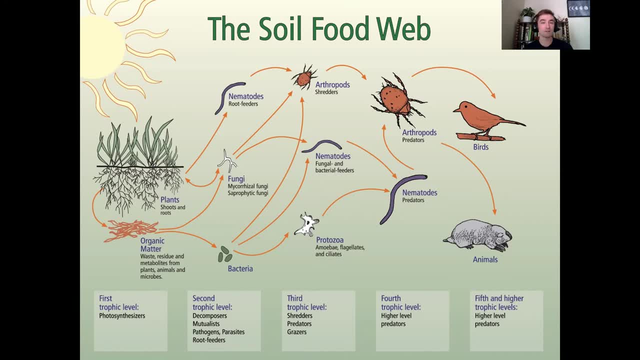 And then you have pathogens, parasites, root feeders and mutualists that will eat the living plant material. These are important because they're the recyclers of the soil. They take all the dead, decaying matter, animal and plant material and turn it back into organic matter or humus. 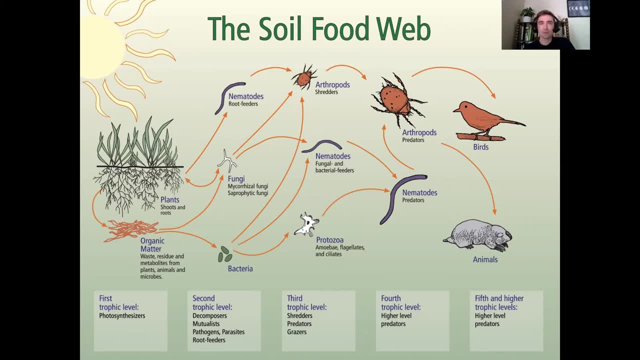 Now, in order for your soil to be really healthy, you need to have a lot of decomposers. In order to have a lot of decomposers, you need to have a lot of organic matter in the first place, But it's not until you get to the third trophic level. 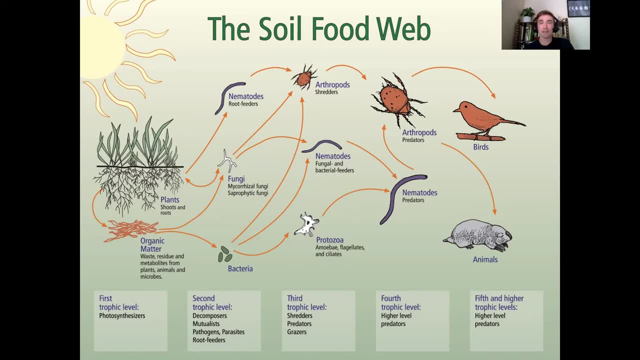 That you start to see the real results of having a living soil. The third trophic level are like the predators of the soil. These are things that are going to eat the bacteria, the fungi and then the root feeding nematodes. 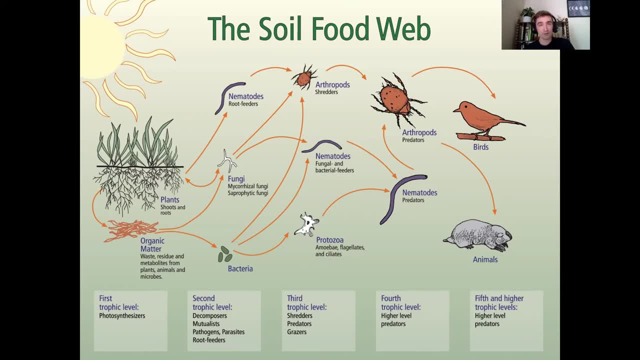 Primarily, these are arthropods, which are little bugs, or protozoa, which is a whole group of organisms That typically are single-cell aquatic organisms. Remember, the soil ecosystem is really an aquatic ecosystem. We have another type of nematodes that will eat fungi and bacteria. 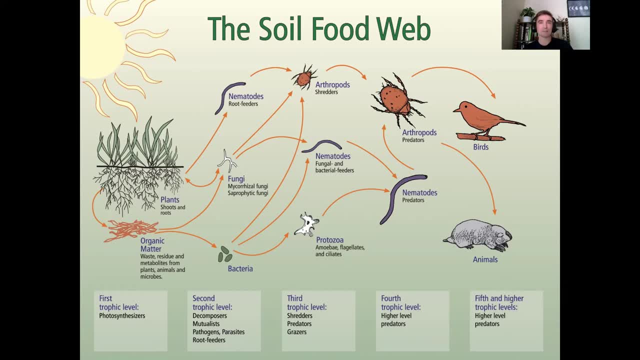 And so it's these organisms that actually release the minerals that the decomposers take into their bodies. So It only becomes available once again to your plant when the bacteria and the fungi are themselves consumed, broken down and then pooped out. 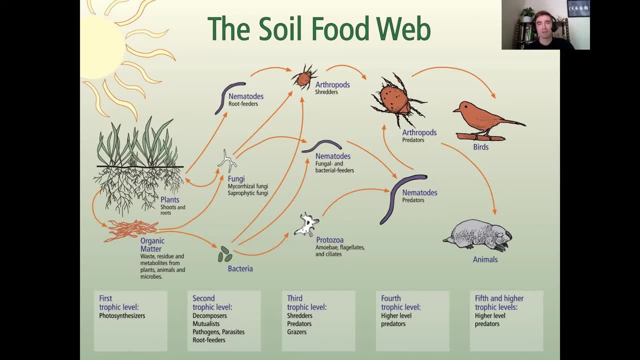 And now everything they ate becomes available And you can imagine you need a lot of bacteria to have enough food, to have some protozoa And even further still if we go up the trophic level. you're going to need a lot of protozoa, arthropods and nematodes. 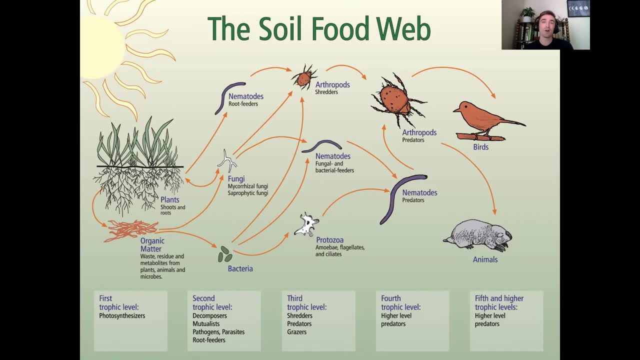 to become The food for the larger arthropods and nematodes, which themselves become food in the fifth and higher trophic level for the birds and the animals that you find in the soil, And so if you see large animals, that's a sign that you have everything else. 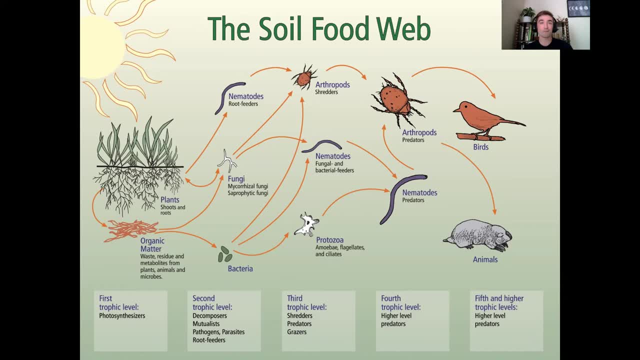 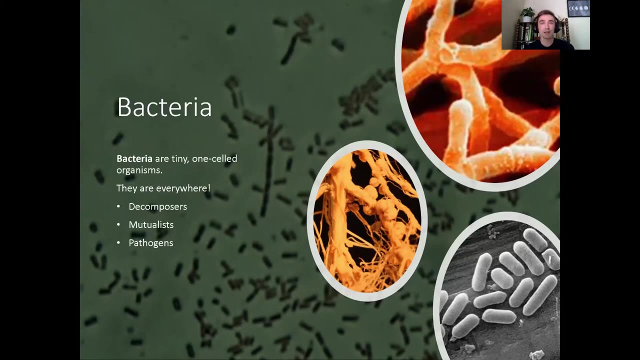 That's a good thing, And it all starts with that first trophic level. You need plants and you need organic matter to be in the soil to build The foundation for the soil food web. Let's take a look at our first category here of bacteria. 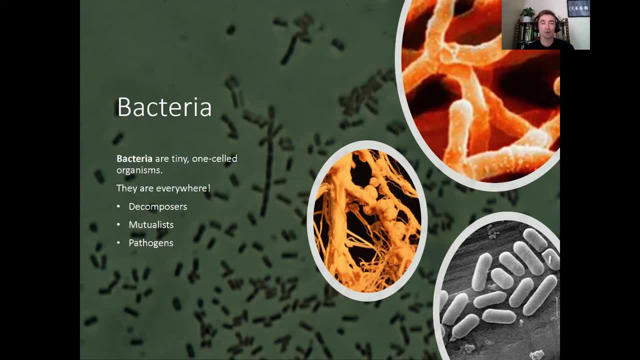 Bacteria are tiny, one-celled organisms. They are everywhere. It has been said that this is a bacterial planet Because they are the most numerous organism on the planet. They're quite literally everywhere. They're all over the place. they're inside you, they're on your skin, they're in the atmosphere. 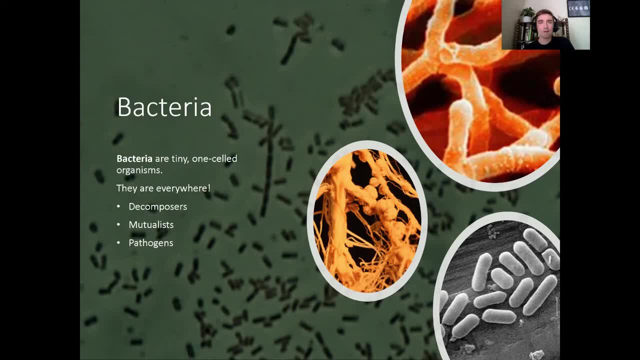 They are found everywhere. They can have many roles. We talked about them being decomposers. They can be pathogens, As you know. some bacteria can get you sick and get your plants and animals sick. And then there's mutualists, where they may form a symbiotic relationship with another organism and work together. 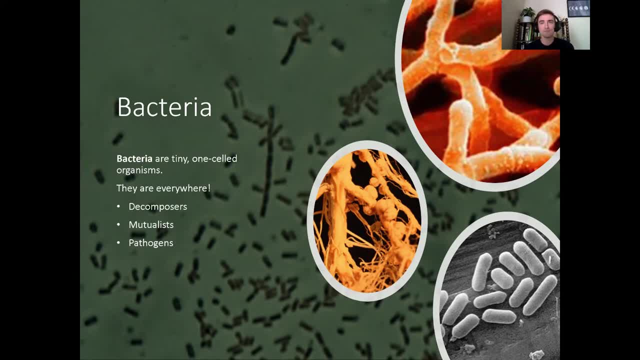 As we'll discuss. The images you see are different types of bacteria And they're easy to identify on a general level. So in the background image, as well as in the lower right-hand image, we see Bacillus. Bacillus is rod-shaped bacteria. 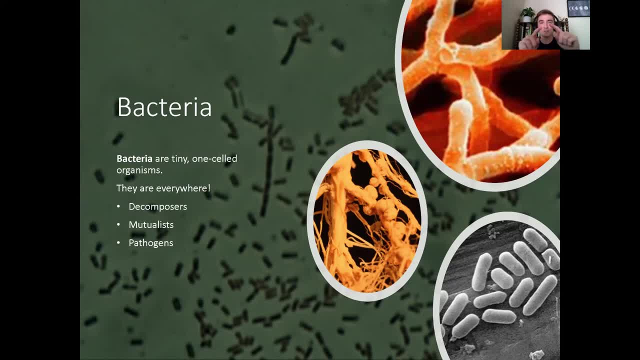 And it's usually like if you took two circles And you put them together, And you put them together, And you put them together And you get kind of like a medicine pill or something. A pill shape, That's Bacillus. If it was one circle all by itself, that's Coccis. 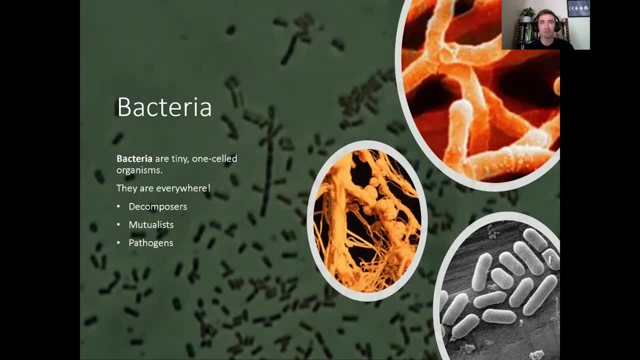 Or if you pluralize them, you'll see Cocci and Bacilli, And those are two general categories for bacteria. The next photo, in the middle, in the oval, you see roots. The next photo, in the middle, in the oval, you see roots. 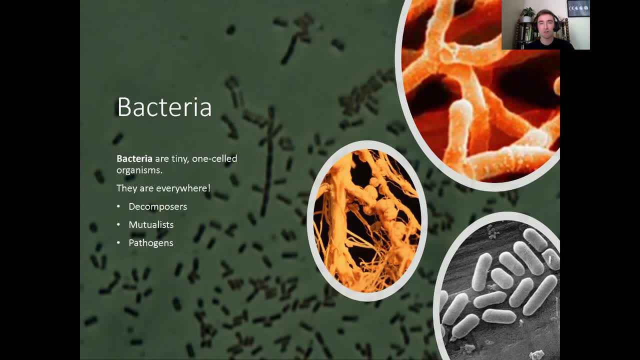 Those are plant roots with little nodules. The growth that's on the roots And the nodules are a house for bacteria, A special kind of bacteria that the plant builds a house for and invites in, And that bacteria is called rhizobium bacteria. 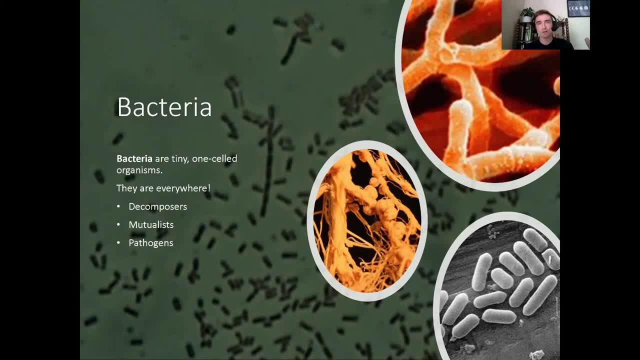 And inside is a bacterium that will take in nitrogen from the atmosphere and give it to the plant in exchange to the plant, in exchange for sugar from photosynthesis. So that's an example of mutualism And there are many examples of pathogens and E coli and salmonella and things. 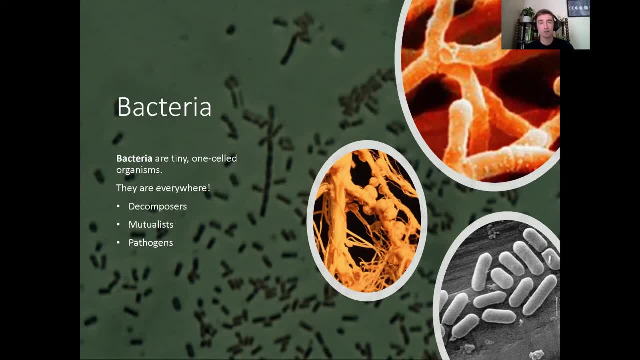 like that are good examples. So bacteria are quite literally everywhere. You yourself are made up more of bacteria than human DNA. So if you could separate out the bacteria from the human and put them both on a scale they say the bacteria weighs more, And so you want to. 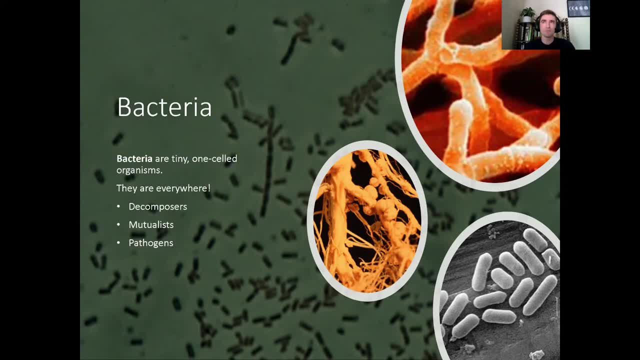 encourage all kinds of bacteria because the more diversity you have, the more balance you're likely to have. If you try to kill off bacteria with some type of sterile or hypoallergenic type of treatment, there's a good chance you're only going to invite in the most aggressive. 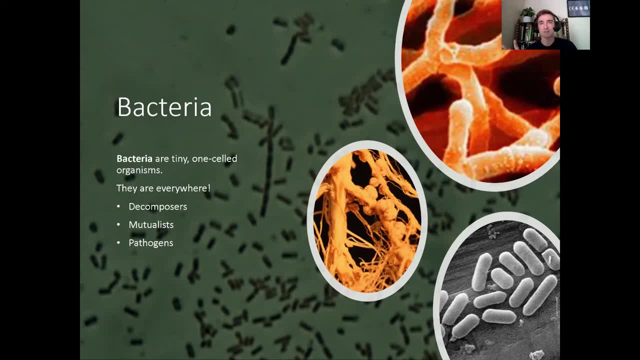 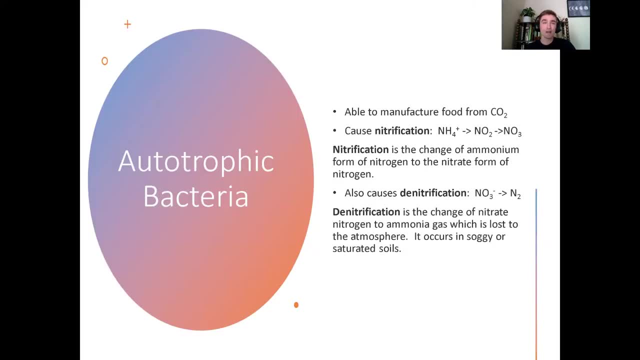 aggressive types. So if we just encourage all kinds of bacteria, then we can have a nice healthy balance, a good diversity Of our bacteria. there are a few general categories and one of them are the autotrophic bacteria, And talking about trophic levels you can probably 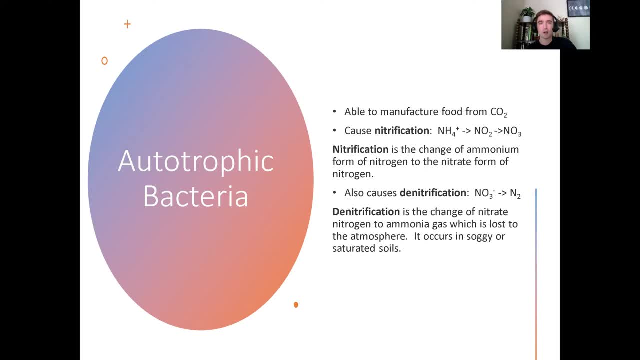 guess that it refers to food, And autotrophic therefore means they can manufacture their own food, And so autotrophic bacteria are the ones that are the most aggressive, And so autotrophic bacteria are the ones that are not aggressive, And so these types of bacteria can take in carbon dioxide and 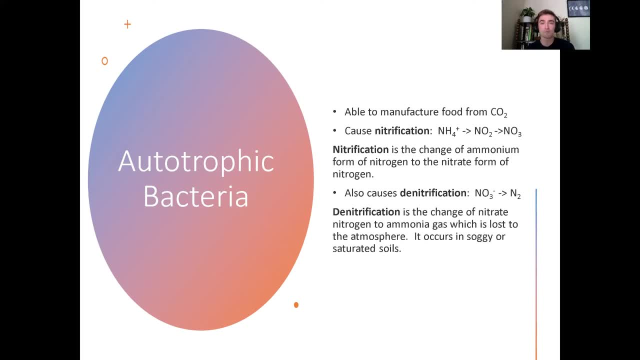 make their own food, very similar to plants. In the process, they end up participating in the nitrogen cycle. So this process for bacteria is called nitrification, And what they do is they change nitrogen from different from one form to another, And typically they're part of the process of making the nitrogen available to your plants. 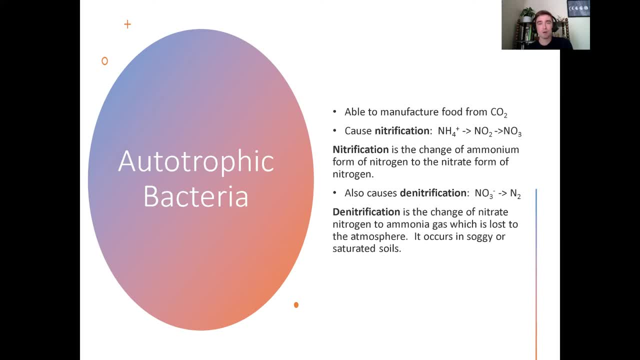 So the process of nitrification is taking ammonium and turning it into nitrite and nitrate, which then becomes available to your plants. This happens in the water. If you've dealt with aquariums, you have to worry about dealing with nitrates that build up. 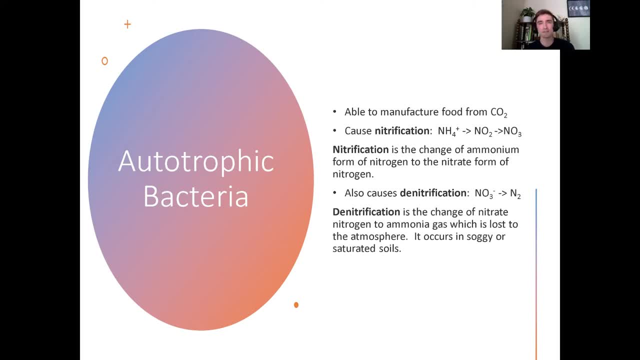 This happens in the soil as well And it's part of what makes nitrogen available to your plants. And there are other bacteria that cause denitrification. that will take the nitrate and turn it back into nitrogen gas or ammonia, And this happens typically without oxygen. 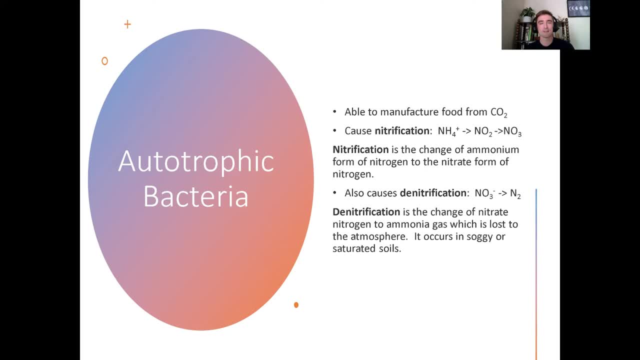 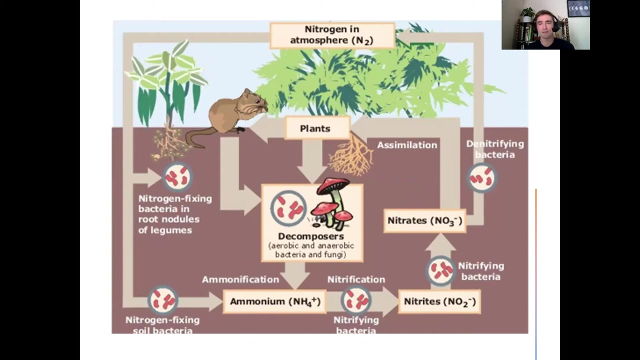 So if your soil gets saturated, You'll have nitrogen being lost. If your soil is filled with oxygen, you'll have an aerobic bacteria that will actually turn atmospheric nitrogen into plant-available, water-soluble nitrogen. Here's a diagram that's illustrating the nitrogen cycle. 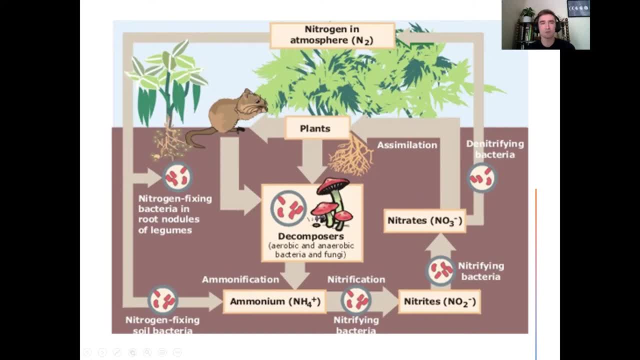 So you can see, in the atmosphere nitrogen exists as N, N2.. And it's the most abundant element in the atmosphere. The vast majority of what you inhale when you breathe air is nitrogen. It's not oxygen. Nitrogen goes down into the soil because there are air pores. 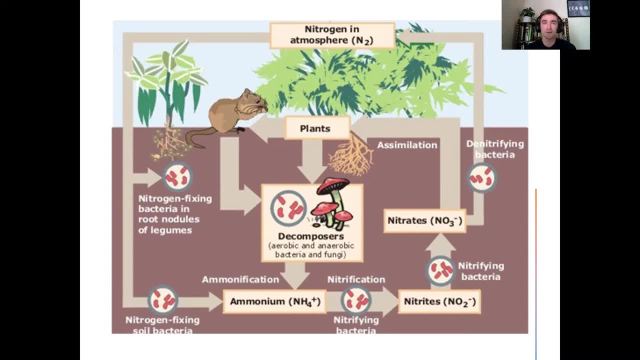 The macropores bring in the atmospheric gas, And so nitrogen is around the roots of your plants. But your plants cannot take up N2.. They cannot get the nitrogen from the atmosphere. That nitrogen needs to be transformed, And so for some plants that have the beneficial relationship with the rhizobium bacteria, 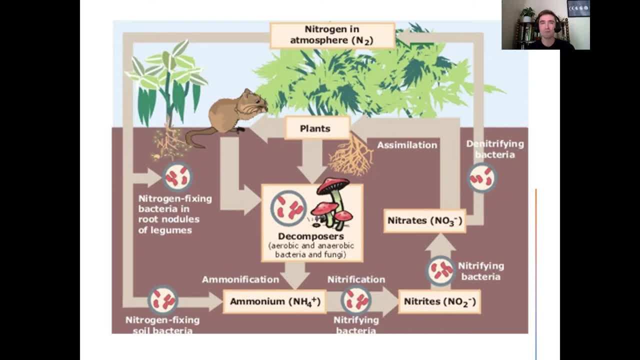 They build the house and the bacteria does that job for them. Those are all your bean plants, legumes For all the other plants. they need to get their nitrogen from autotrophic bacteria. They need to get their nitrogen from autotrophic bacteria. 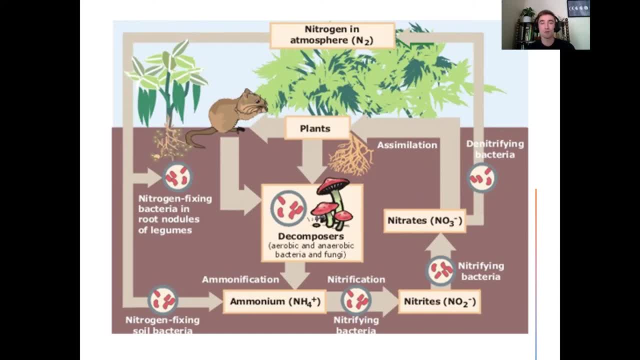 that can transform N2 into ammonium nitrites and then nitrates, And notice there's different species of bacteria that participate in that entire chain. Once it's in nitrate form it can become water-soluble and taken in through the plant's roots. 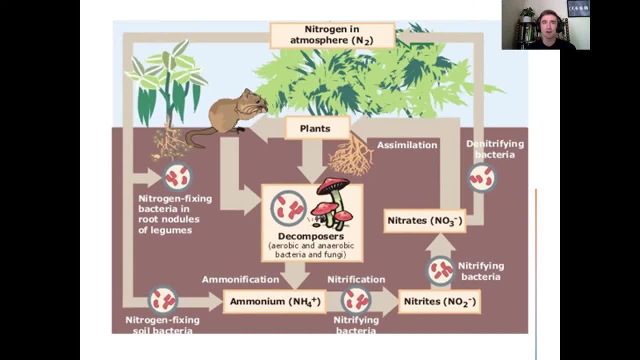 kind of like a smoothie or like a juice. It's got all the minerals in it but it's in liquid form. And then, once those plants die and decompose, either the animal will eat the plant and then get rid of it as manure. 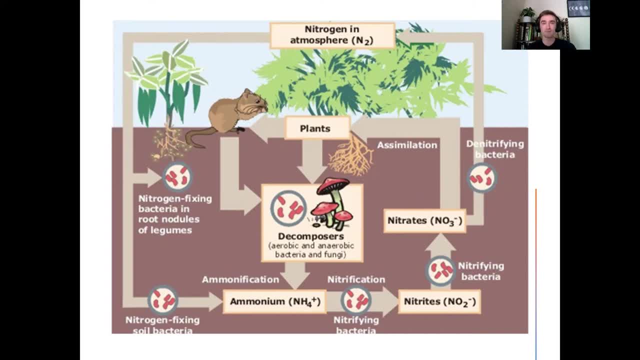 or the plant itself will fall and die. There's still nitrogen in those leaves and in that manure, And now we have the decomposers, which are different types of bacteria and fungi which break down the nitrogen in the animal and plant material, the organic matter. 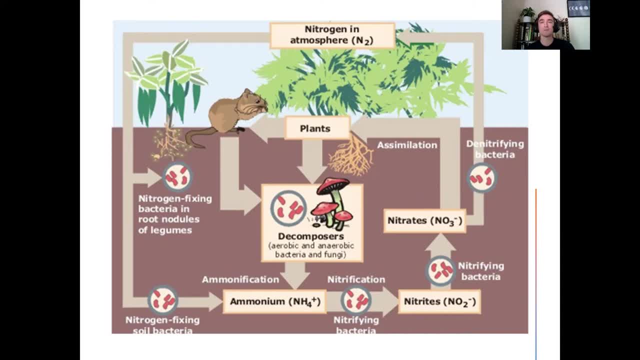 and convert it back into ammonium so it can go back through the cycle. So if we have organic matter, we can have decomposers and we can hang on to a lot of nitrogen in the soil. Otherwise, what's going to happen is it'll have to go back up into the atmosphere. 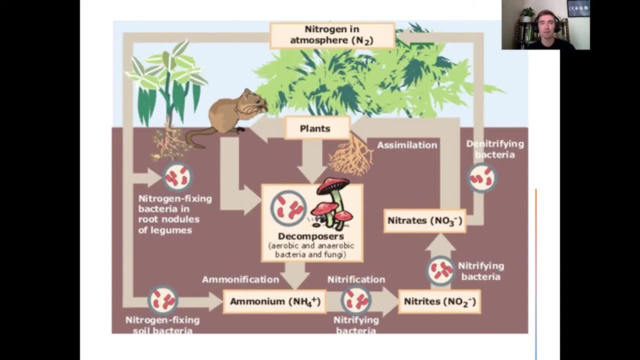 and it's one less pathway for the nitrogen to be brought in available to your plants. So this shows the importance of You have the decomposers and the organic matter in the process. Otherwise you have a lot less nitrogen to go around, literally to go around the cycle. 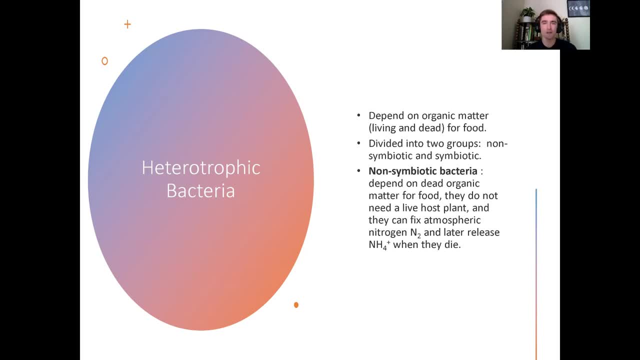 And the next type of bacteria is called heterotrophic bacteria, And these are those decomposers. These are the ones that depend on organic matter- living and dead- for food. And there's two main types of heterotrophic bacteria: things that need to eat other things. 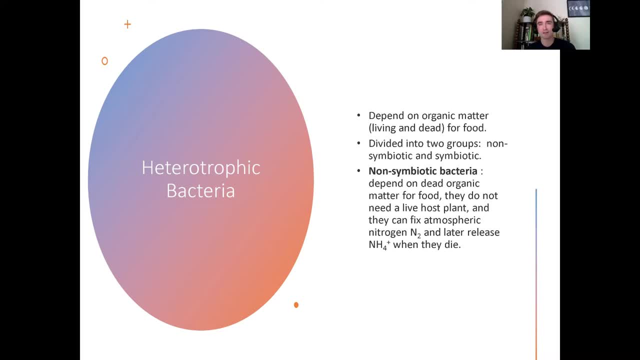 There's symbiotic and non-symbiotic. So the non-symbiotic is something that lives all on its own and can go out and find something to eat, So it just eats dead organic matter for food. They don't need to be tied with a host plant. 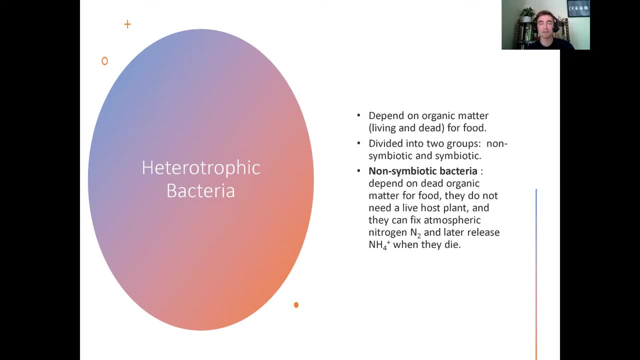 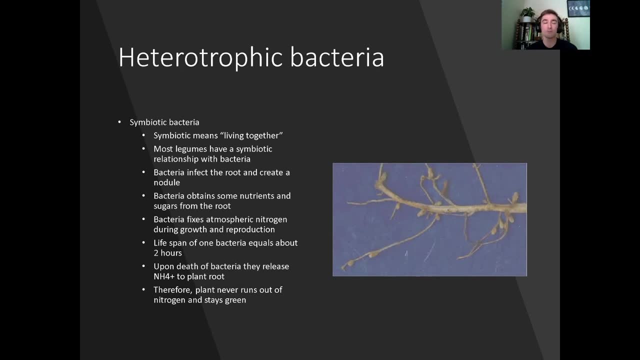 So these are the majority of the decomposers, the things that are living in a compost pile, for example, And then the other type of heterotrophic bacteria is a symbiotic bacteria, And this is that root nodule that is found on our legume plants. 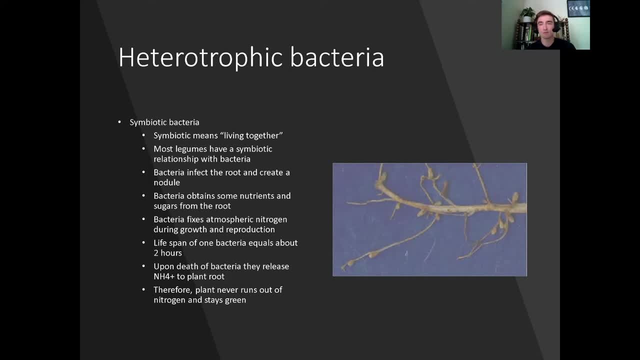 It's called rhizobium bacteria. And those little nodules, those little bumps on the roots, those are rooms that the root created to invite in the bacteria, And the bacteria will then live inside And be able to take in nitrogen from the atmosphere. 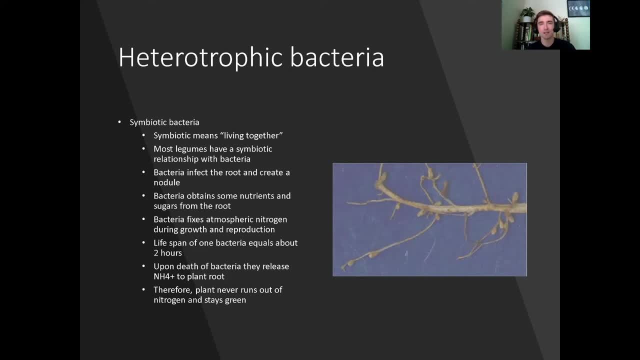 give it directly to the plant And the plant in exchange gives part of its sugar from photosynthesis in to the bacteria. They both get what they need by working together. There's another group of plants related to alder. It's a type of tree. 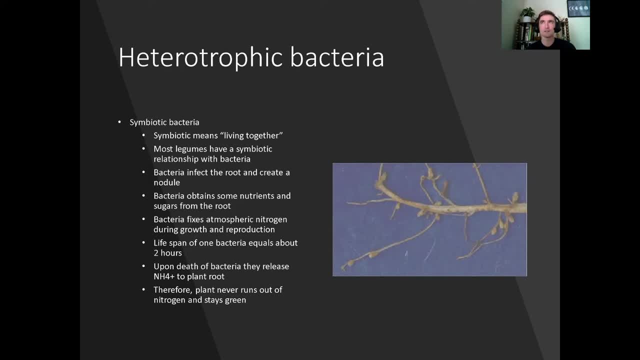 And we have ceanothus in San Diego as a native plant. that is a native plant, That is not a legume, But they have a similar relationship to a symbiotic bacteria that lives in root nodules And it's not called rhizobium. 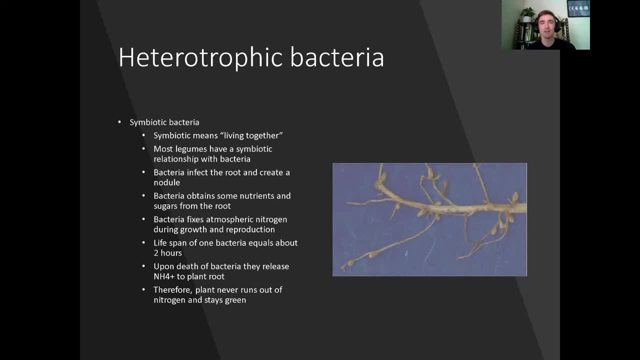 Instead, it's a totally separate evolution, And the name of that bacteria is francia. So francia live inside of alder trees, And then rhizobium lives inside of all of the legumes. Everything else, Everything else needs to find its own nitrogen. 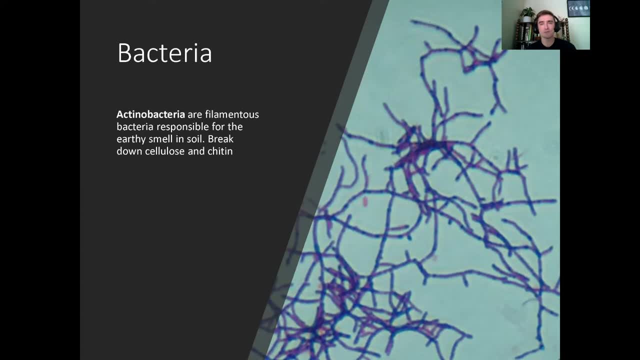 There's a unique type of bacteria that used to be classified as a fungus because of its thread-like nature. So recently, though, it was studied in greater detail And they discovered. you know what? This is more like a bacteria than a fungus. 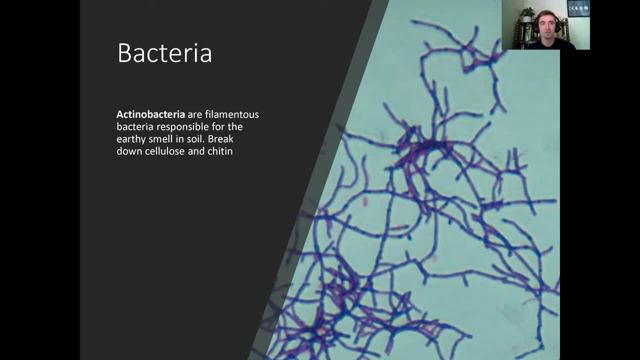 And so now we have this special type of unique filamentous bacteria known as actinobacteria. They used to be called actinomycetes, Now they're more properly called actinobacteria, And if you go to a microbiology conference, 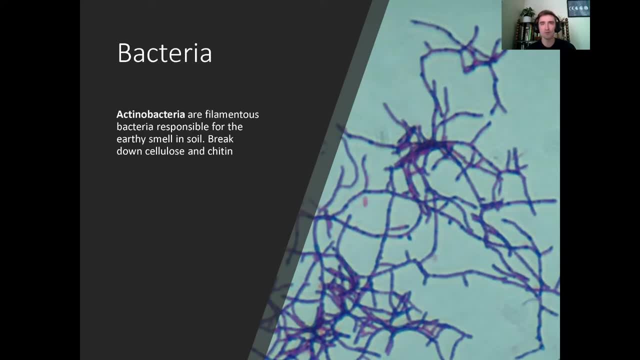 you can witness the arguments between those who think they should be called actinomycetes and actinobacteria. It's a heated debate. It keeps people up at night. What to call these things, And I don't care what we call them. 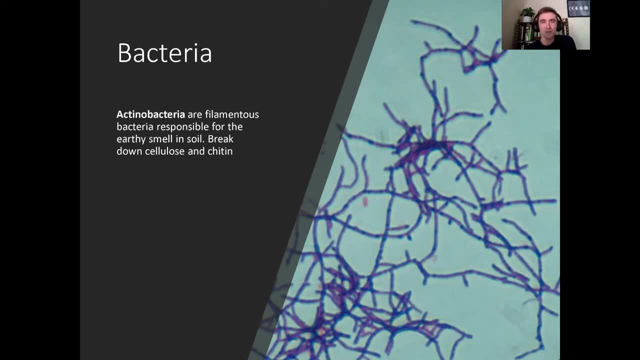 And the organism doesn't care what you call it, But it's important for us to keep learning so we can try to understand these better. These actinobacteria have a crucial role in decomposition. They're part of the reason that healthy soil filled with humus 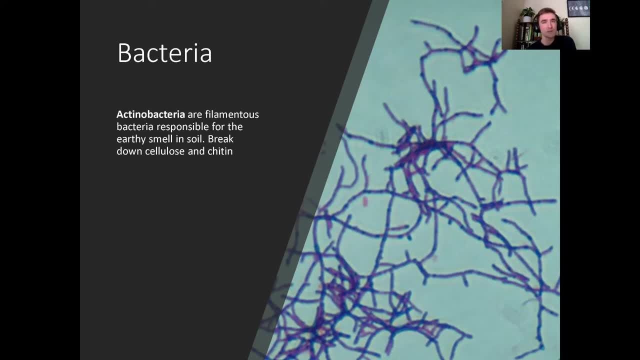 smells like that rich, earthy, sweet smell that everybody likes And everybody knows it smells good, because our ancestors needed to know that that was healthy soil. So actinobacteria are responsible for that earthy smell in soil and they have the ability to break down cellulose. 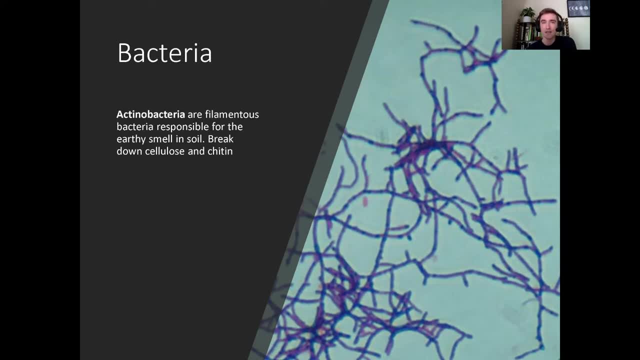 and chitin, And chitin is the exoskeletons of bugs And it's the mycelium of fungus. Not many other things can break that down, And chitin is very similar to your fingernails and your hair. Actinobacteria smells like a meat. aphid İns %b. Etc è 氣. so actinobacteria is the material that surrounds a fungus, The mycelium of fungus. Not many other things can break that downON, and chitin is very similar to like your fingernailsThey've been this product. Da voz de So, paula nas qued duty paraE. today I haven'gestellt. 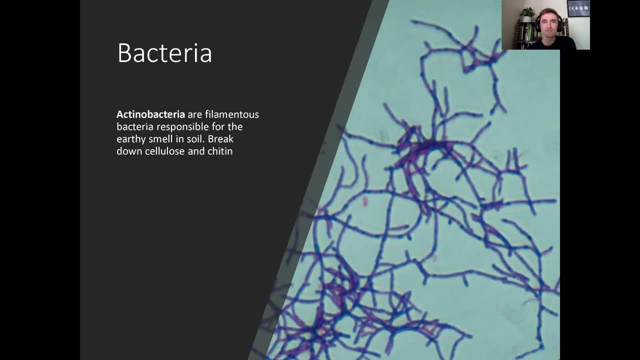 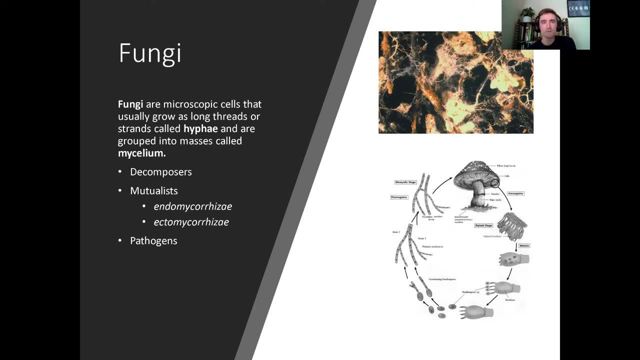 Echinobacteria can break that down too. So let's take a look at fungi, and you can pronounce it fungi, fungi, fungi, however you like, Although most scientists, I believe, call it fungi- That's the plural- A single is fungus. 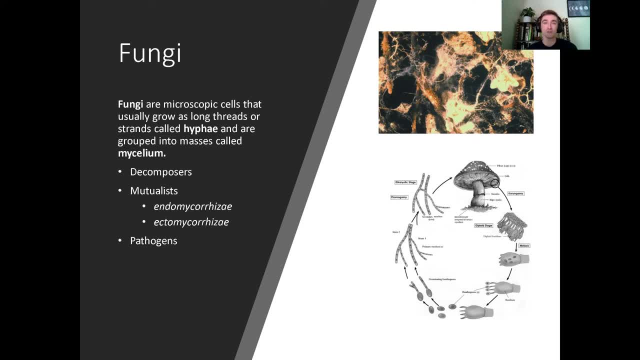 So fungi are microscopic cells that usually grow as long threads or strands. The name of those strands are hyphae And those are grouped. when you get a bunch of strands put together into a web. that web is called mycelium. That's the real fungus is this web of mycelium? 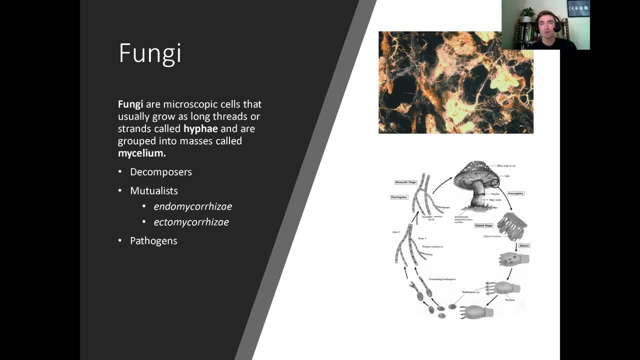 Cells, mycelium. When we think of fungus, we typically think of mushrooms, But mushrooms are kind of like the apple of the apple tree. So the mycelium is the organism, That's the thing that's living and going through all of the biological processes. 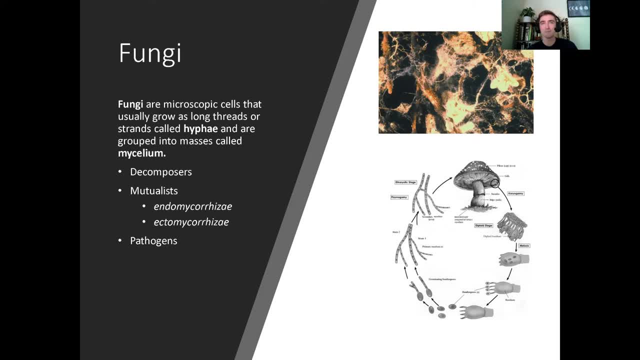 And when it's time to reproduce, that mycelium will send up a fruiting body And we call that a mushroom. So the mushroom is only the attempt to reproduce. The mushroom goes up, it releases the spores out into the atmosphere and into the environment. 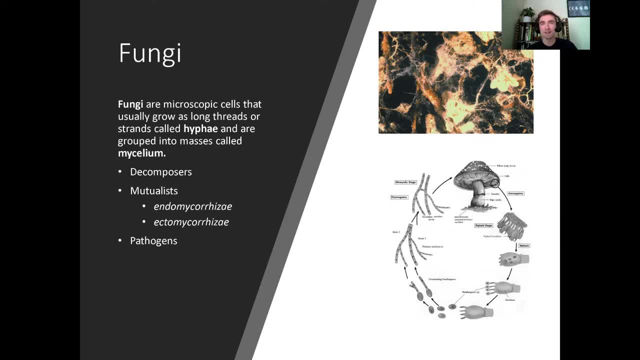 And then they travel wherever they do and they'll land and hopefully form a new colony of mycelium. But really you can pick a mushroom over and, over and over and you'll never get rid of the fungus. The fungus lives in the soil. 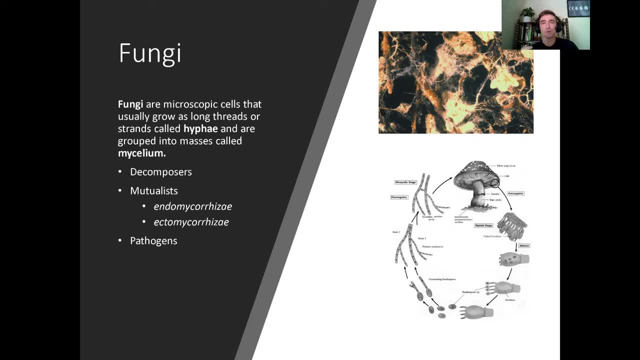 Fungi are primarily decomposers, but there's also pathogens among them as well. So traditionally, horticulturists were mostly concerned with the pathogens. And let's kill the fungus antifungal. Let's get rid of the pathogens, which is still worth doing. 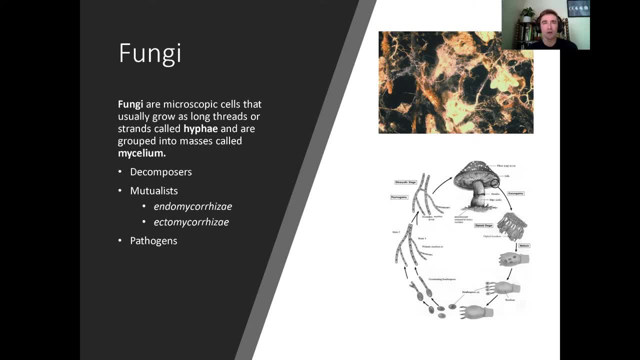 But now we have a newfound approach for soil health and ecology, And we want to encourage the decomposers as well, And that's why we're doing this, And that's why we're doing this, And that's why we're doing this. 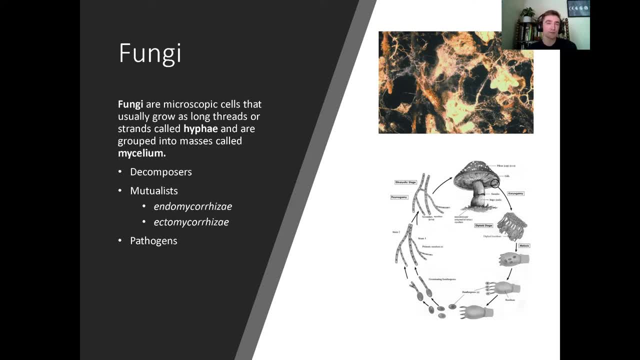 And then there's that other category of mutualists, And we're still learning a lot about mutualisms between plants and fungi. But it has come to scientists' attention that almost every plant species on Earth has some sort of symbiotic relationship, beneficial relationship, with a fungus species. 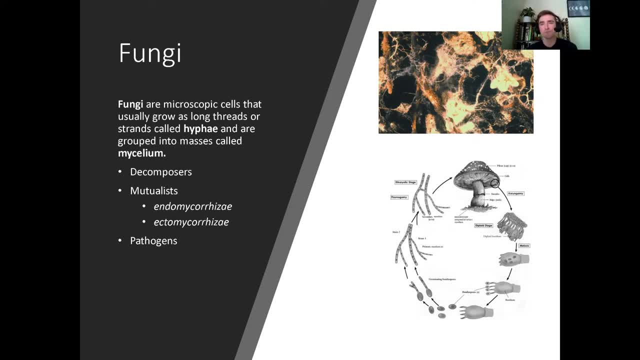 As decomposers in the soil, like the image on the top. fungi have an ability that bacteria do not. Fungi have the ability to decompose lignin. Now, lignin is the woody material found in plants, whereas cellulose is the green herbaceous material typically found in plants. 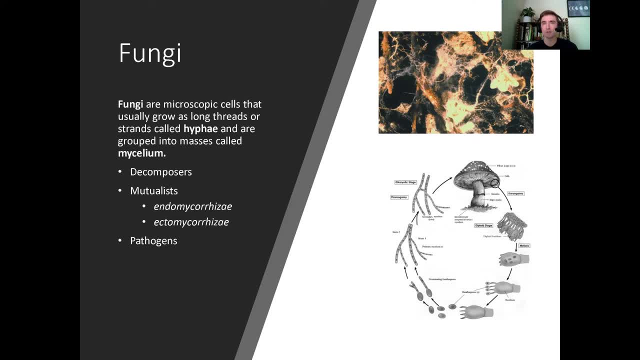 So woody trees and shrubs, things that create wood, they have an extra type of organic compound that's called lignin. That's literally what the wood is is lignin, And nothing can decompose lignin except fungi. Do you know anything else that can eat wood? 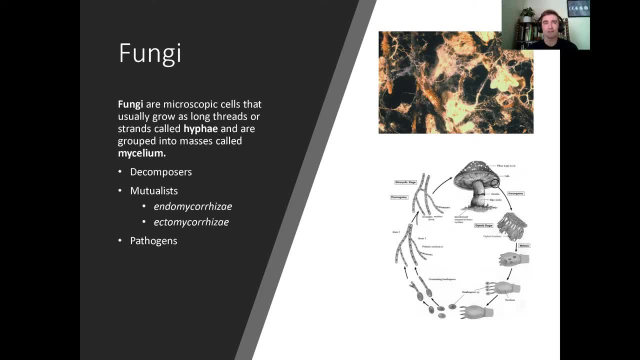 Well, how about termites? Termites eat wood, right? Well, termites, they have a special digestive system, And inside the termite lives the fungi, And so it still is fungi That decomposes lignin, no matter where you go. 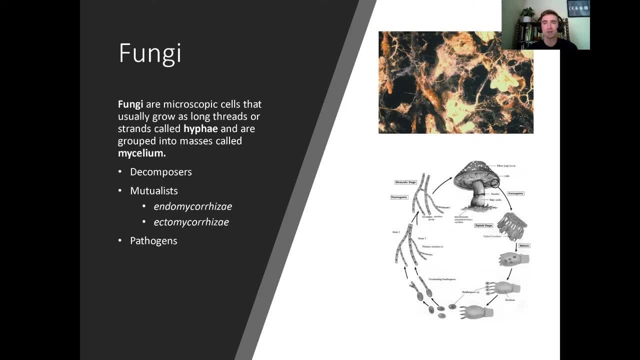 And so we should be thankful to fungi, because without them we'd have logs built up all over the earth. They are what can turn wood back into soil. When we look at the mutualists, we have the ability for these fungi to connect to the plant roots. 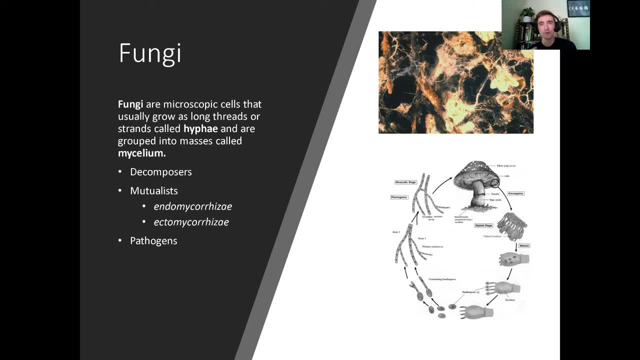 And what happens is they will team up with the roots of, say, a tree, and they will extend the functionality of the root system And they can even connect multiple trees together. And so, just like with bacteria, the tree will give the fungus some sugar from photosynthesis. 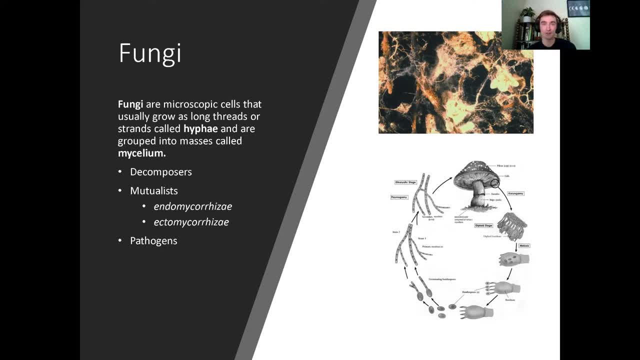 some of the sweet sugar, the calories, the energy And in return, the fungi will give the tree more water and more nutrients. And this web, this mycelium in natural ecosystems, has been compared to the internet as sort of an analogy. 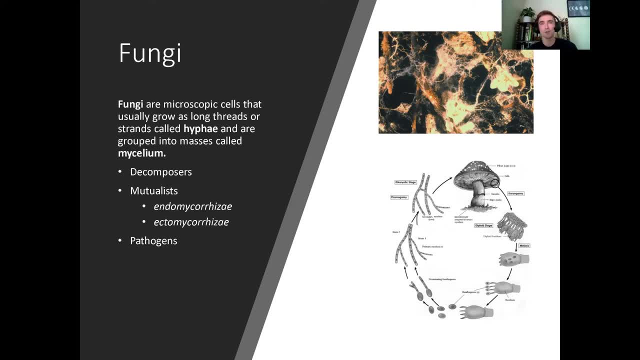 Just how you can go on the computer and be connected to other people all over the world and spread information. The mycelium in an ecosystem will connect multiple plants and multiple species to each other, And if one has extra sugar, the fungi, the fungus- can actually take that from the roots. 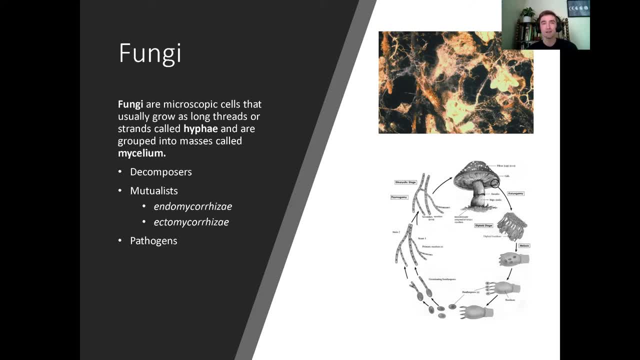 and give it to another plant. And so some of these plant species in true wild ecosystems they don't grow very well by themselves, They kind of need to be, they need to be plugged in to a network. And what is the network? 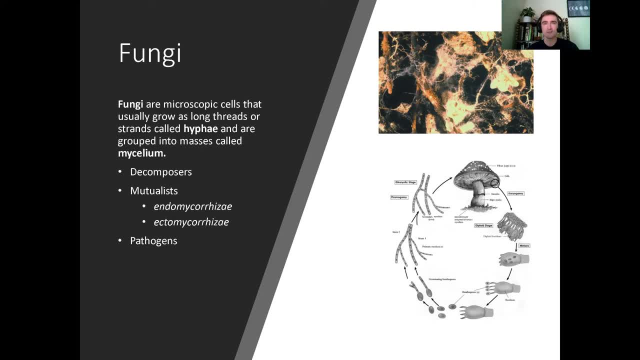 It is literally a fungus, a giant fungus, And the largest organism on the planet is actually a fungus, And it can stretch for many miles And some scientists were taking samples and they were doing DNA analysis And they said: you know what? 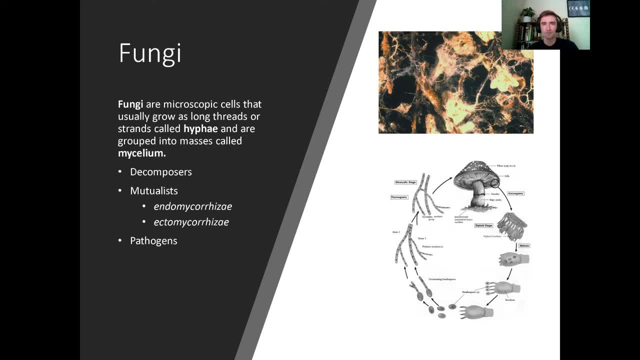 This isn't just the same species, This is the same individual, And it's over this huge area, And it can spread larger than some US states, And so, even though it's mostly invisible to us, it's the largest known living organism on planet Earth. 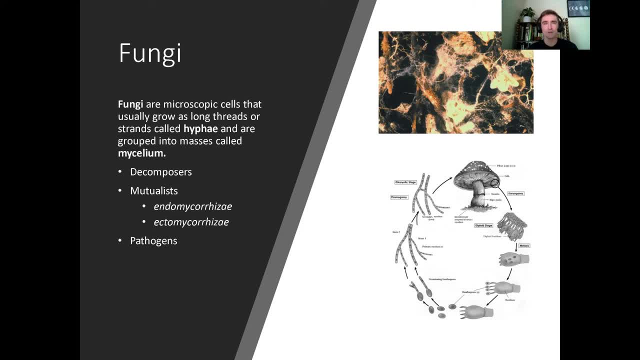 is one individual of a fungus. And so there you go. It's a mutualistic fungus. Of the mutualists, there's two different ways they can partner with plants. They can be endo Or they can be ecto, And so that's literally just like a USB or another type of connection. 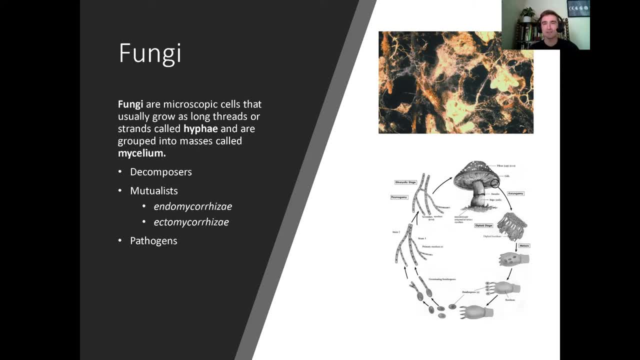 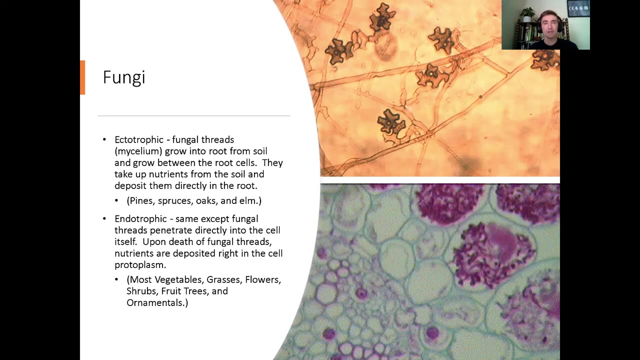 And so how do you want to plug into the internet? And different plants will have endo associations, Others will have ecto associations, So the ectotrophic fungi. they connect to your plant roots By growing in between the root cells, So they just have a little mechanism that enables them. 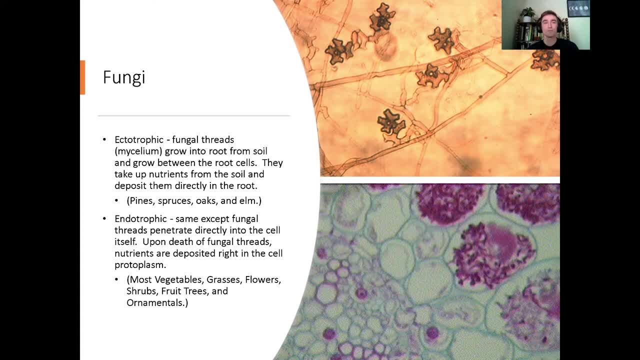 to squeeze inside and go in between root cells And they'll take nutrients from the soil and they'll deposit them inside of the root, right for the tree, like a little gift, And in return the tree gives sugar. So these are pine trees, spruces, oaks and elms. 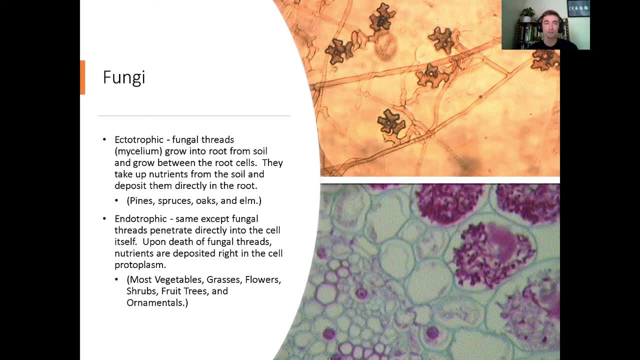 So these are pine trees, spruces, oaks and elms, Those four types of trees. they are ectotrophic, meaning they are looking to plug in with ectomycorrhizae or mycelium that are going to plug in between the root cells. 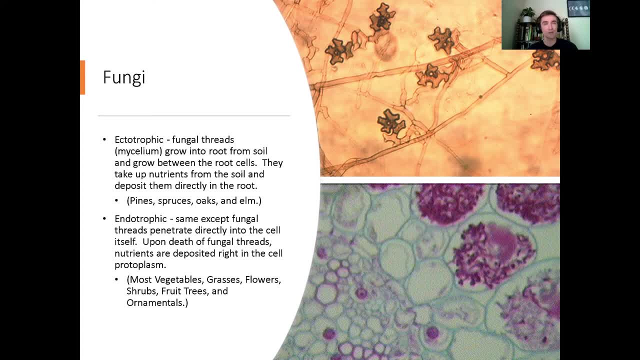 The other type, which is most of the other plants that have fungal associations. those are endotrophic, And what that means is, instead of going between the root cells, here the fungal threads, the hyphae, will actually penetrate the cell itself. 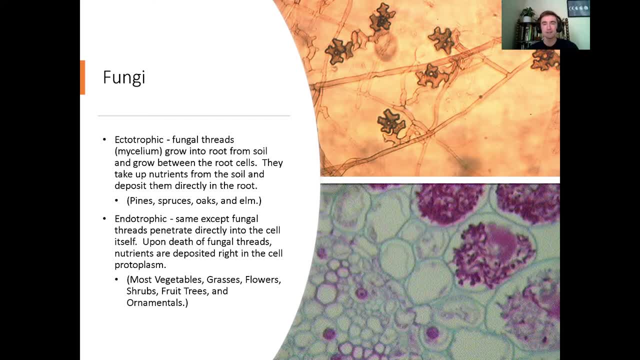 and live inside the cell, And that's what the bottom image is showing- is the fungus inside the cell, And so, then, the fungus that's in there will die periodically. It's always growing and dying, And as it dies it releases nutrients right there inside of the cell. 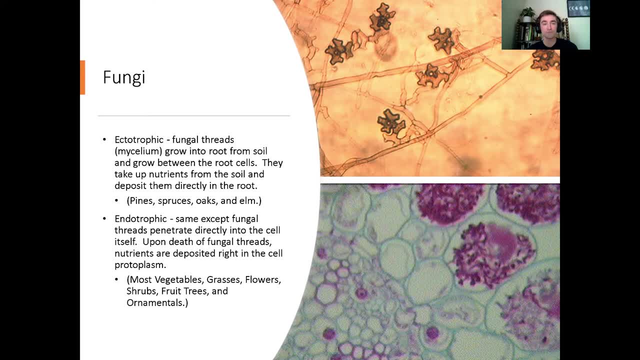 So most of your vegetable crops, most of your grasses, your flowers, your shrubs, your fruit trees, most ornamental plants, most native plants. even in San Diego you don't think we have mushrooms, but we've got a lot of fungus in our soil. 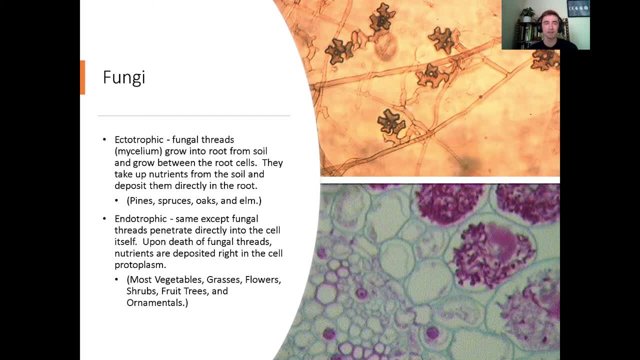 Most of them are endotrophic: the plants themselves and the fungi are endomycorrhizae. If you are in a nursery and you want to add some mycorrhizae, which is basically root fungus for your plants, you need to know. 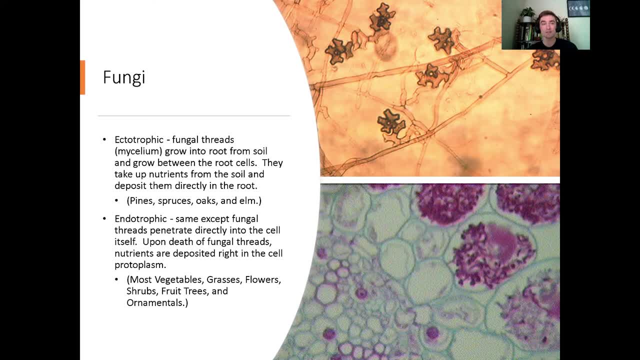 are these ectotrophic or endotrophic? So it makes no sense to try to put ectotrophic mycorrhizae on endotrophic plants. So most of the time, if you buy mycorrhizae as an additive to your potting media, 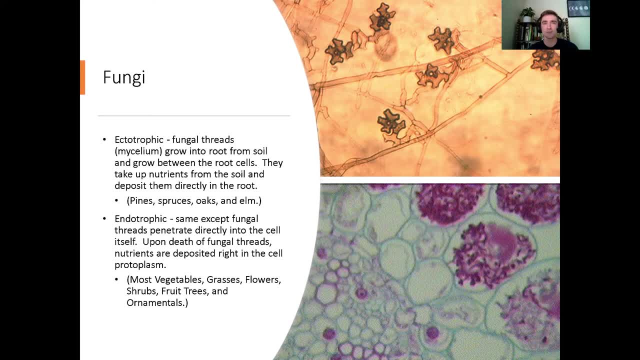 it's going to come with a little bit of both and you need to grow it first before you add it, But I have seen it produce very positive results. Some of the few types of plants that have no associations with fungus are anything related to cabbage or broccoli. 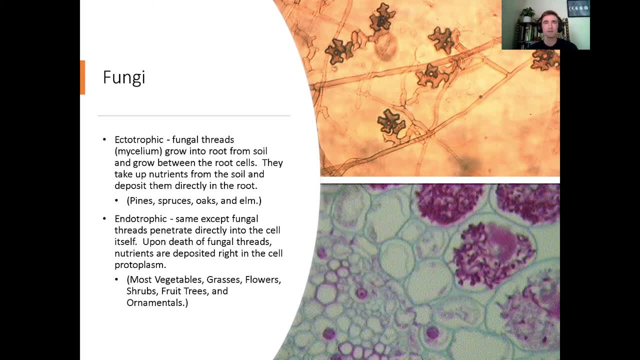 So if it's in the brassica family, if it's kale, collard, greens, Brussels sprouts, mustard, cabbage, broccoli, cauliflower, none of those have any connection to fungi And there's some speculation that they actually discourage fungi in the soil. 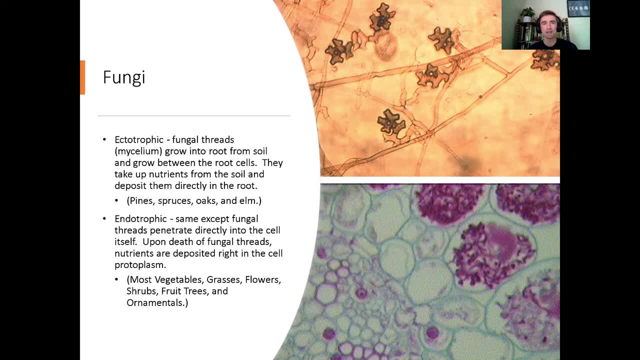 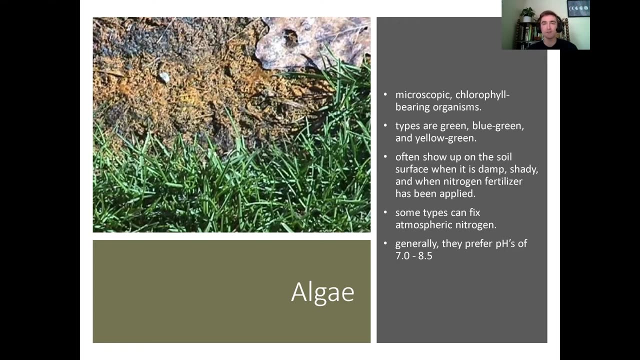 So you typically don't want to plant those right next to other plants that you're hoping to encourage the endotrophic mycorrhizae. Another organism we can have in the soil is algae, So algae is photosynthetic if it's green. 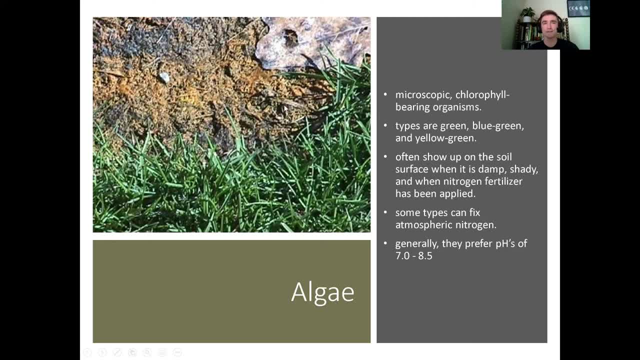 And usually you have algae when your soil is too wet. So if you're overwatering, if there's a break in a pipe and the irrigation is just running all the time, you'll get an algae buildup. Typically that means you have a saturated soil. 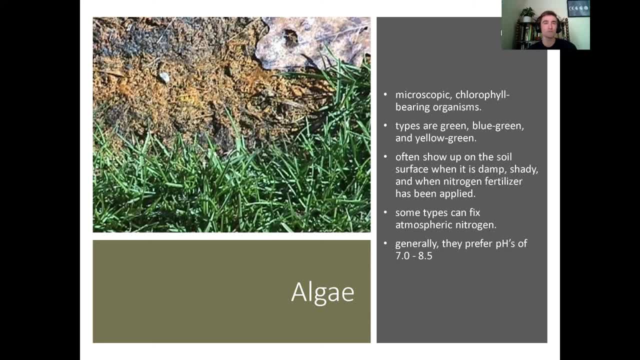 and it can even be a toxic situation for your plant roots and for soil health. So normally you do not want to see algae in your soil. If you do, you can till and turn up your soil and try and get more oxygen in there and then address the problem. 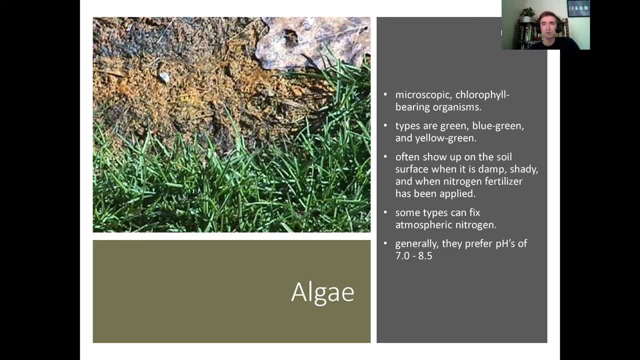 Why was it too wet And what was causing this to build up? Now that's in a cultivated soil, but we have another instance in which algae is present in native, natural San Diego soil and that makes our dry land soil a little bit unique. 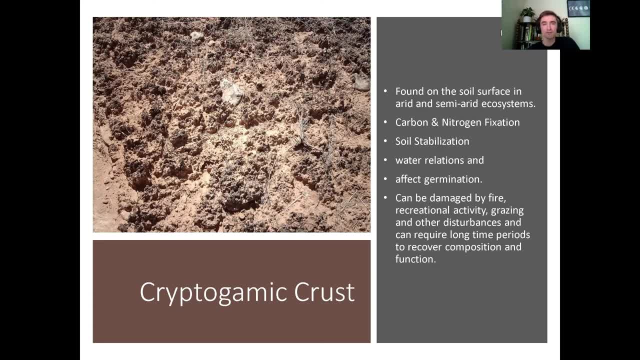 Here in cryptogamic, cryptogamic crust. This is soil that kind of looks rocky, if you didn't know any better, But what it is is it's something that happens in arid or semi-arid areas. We get it in our area. 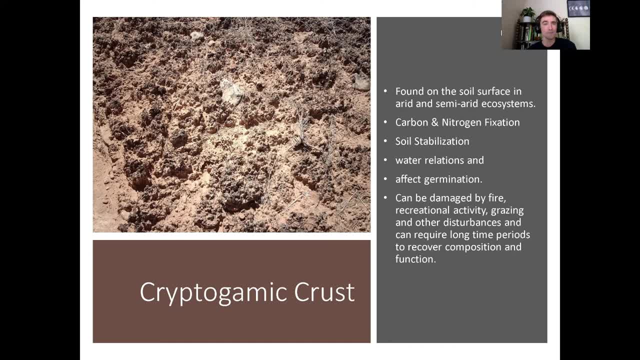 If you don't mess with the soil for a long time, like 40 years, after 40 years your soil can develop this crust. It's called cryptogamic crust And it's actually a bunch of dried up moss and lichen and fungi. 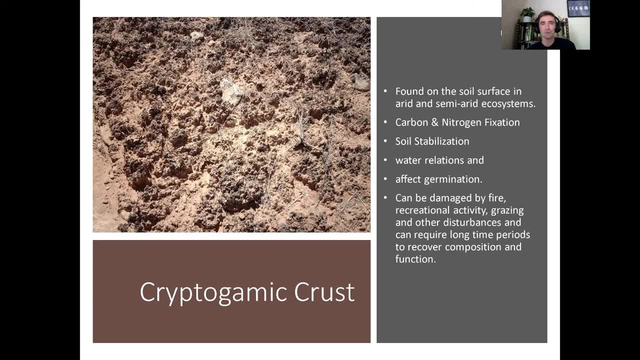 and algae is in there too And you wouldn't think it's anything special. but if you walk on that you can kill it and it'll take you 40 years to get it back. So when you see the cryptogamic crust, 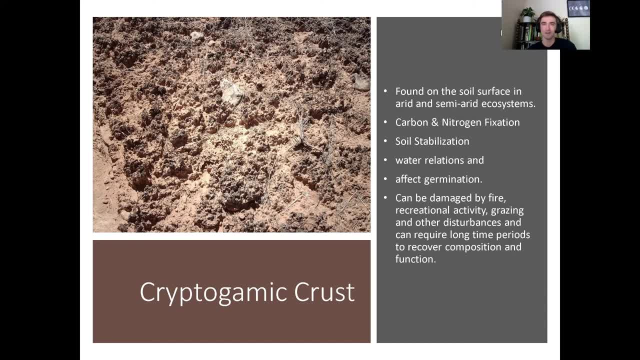 especially in the summertime. don't walk on it. In the wintertime this will green up and turn into a green carpet of moss. You often find it in the shady sides of the shrubs And even on trails. you'll see it on the sides. 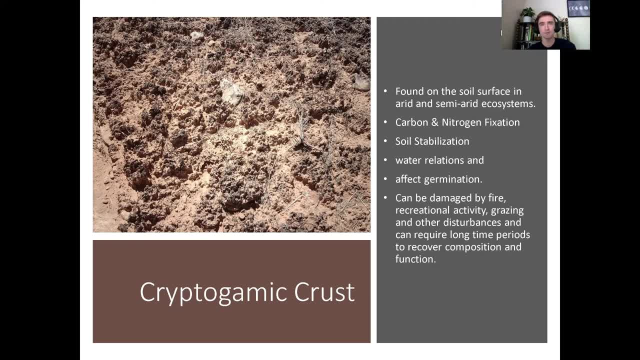 where the trail has been made but hasn't been disturbed. And this cryptogamic crust acts like a mulch. Now, it's not the same as mulch. It doesn't decompose, This is alive, but it traps in the moisture. 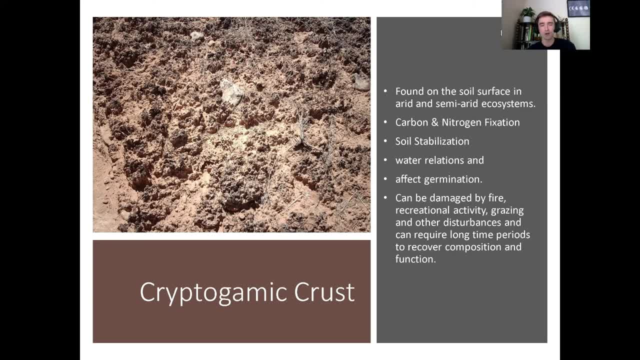 and it's a vital part of the carbon and nitrogen cycles in the soil And it's really essential for your plants to have access to this. So this is kind of the edge of what we understand right now. If you want to get into soil science, 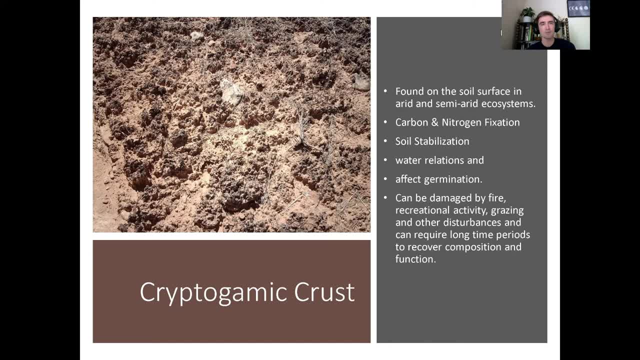 and discover something you may end up wanting: to study this cryptogamic crust and helping us to learn what exactly is it doing and how important is it, and how do we make it and how do we protect it. So it's a really valuable tool. 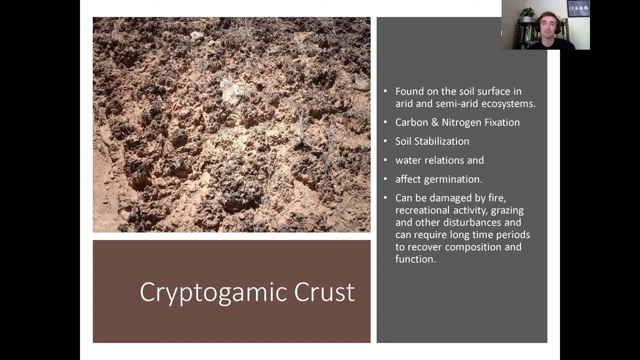 and it can be used to be damaged very easily by fire, by grazing, by disturbance, by many things, And so we want to study it and learn more about it, And when you see it, you have found something special: You've found an undisturbed area. 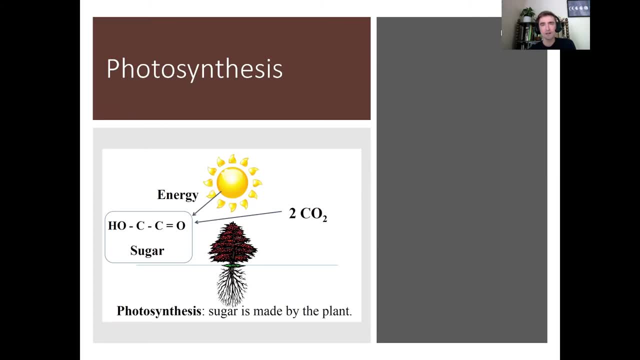 So just to clarify what's going on from a very basic but scientific explanation, remember plants. they are the first trophic level of the soil And so they go through the process of photosynthesis, which means they take energy from the sun and they take CO2,. 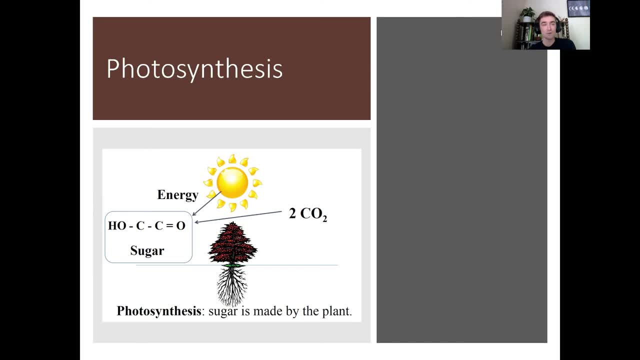 carbon dioxide from the atmosphere. With the presence of water from the roots, they create sugar. And what you see? there is the type of bond, chemical bond, that sugar has. But don't worry about that for right now. Just remember that the sugar 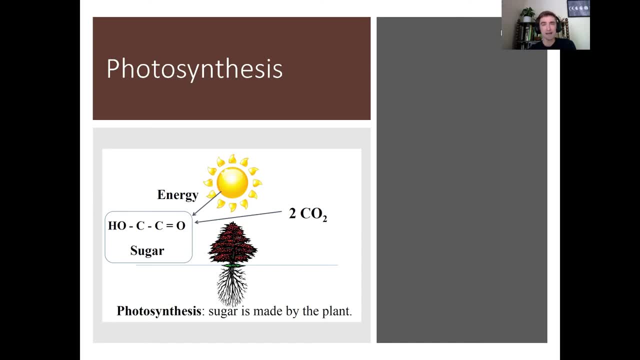 is made by the plant, And that is the calories, That is the energy, That's the food. So plants make their own food. All the other stuff that comes from the soil is minerals, but there's no energy there. The energy comes literally. 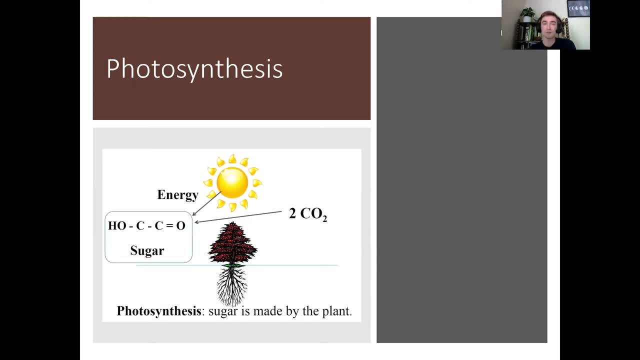 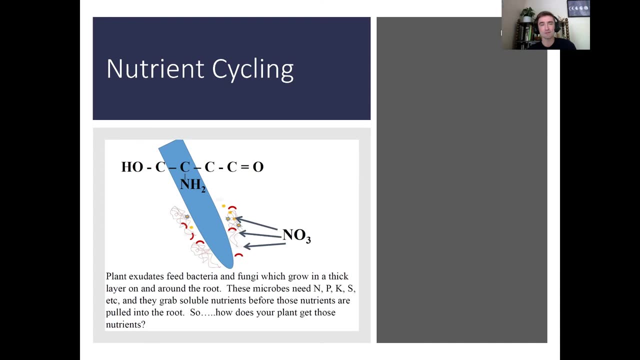 from the sun. The sun is how the sugar is created, And then, in part of these nutrient cycles, the plants themselves will direct the sugar down to the roots And every cell in the plant gets a little bit of sugar because it needs that sugar. 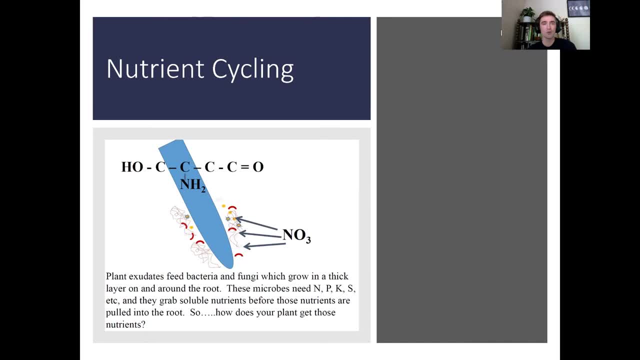 to carry out its functions of living. But anything that's left over and extra gets released by the roots. These are called exudates, because the plant roots will exude this little chemical And this chemical will feed the bacteria and the fungus in the soil. 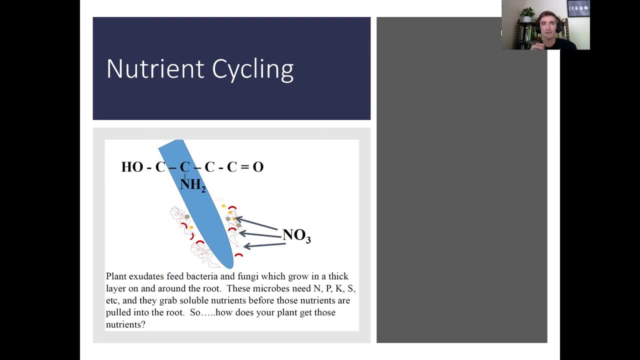 And it ends up growing a thick layer of these organisms right around the roots. So your root system becomes its own little ecosystem. We call that the rhizosphere, So the soil right next to the root is this rich ecosystem of minerals and nutrients that are changing hands. 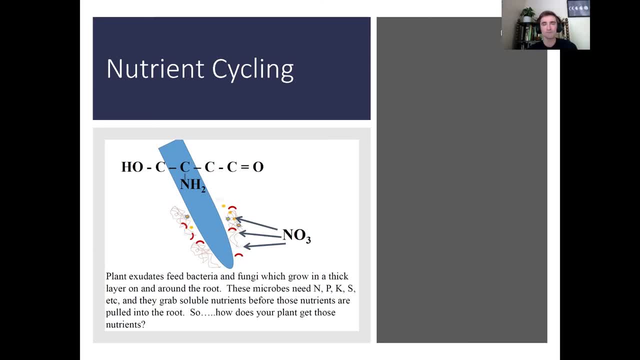 And it's actually quite a quick process. We believe that in a fraction of a second the plant can know that it needs some calcium, And so it'll center it and send out a special chemical from the root that will encourage the calcium bacteria to take in the sugar. 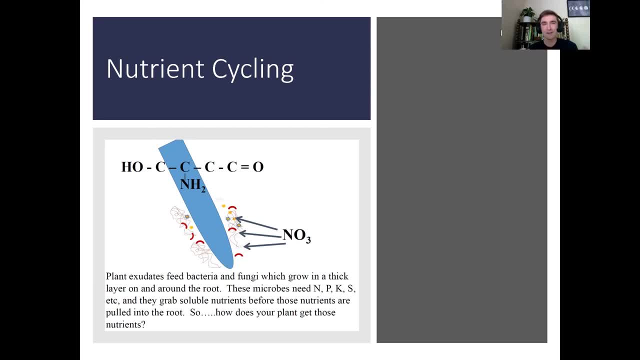 and mineralize some calcium from the soil And within one second the plant can need calcium, feed calcium and then absorb that calcium and direct it to the spot in the plant that it needs it, And we have no clue how that works. 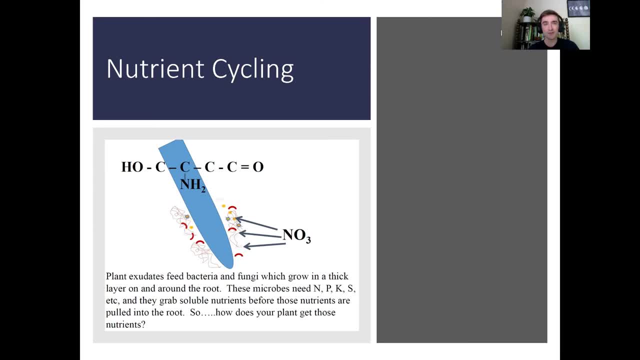 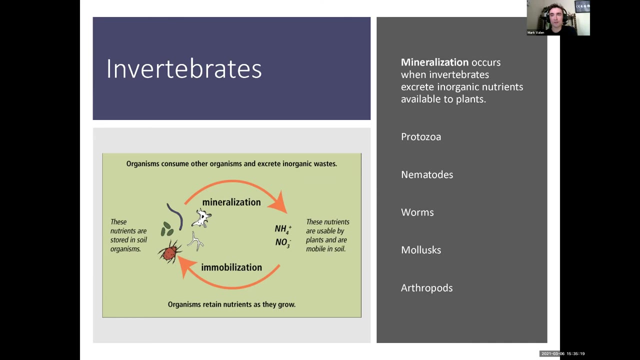 And so, if that is interesting to you, please continue your education and help us understand what's going on here. The plants are kind of cultivating the organisms that they want when they want them, So this is where the process gets a little bit tricky. 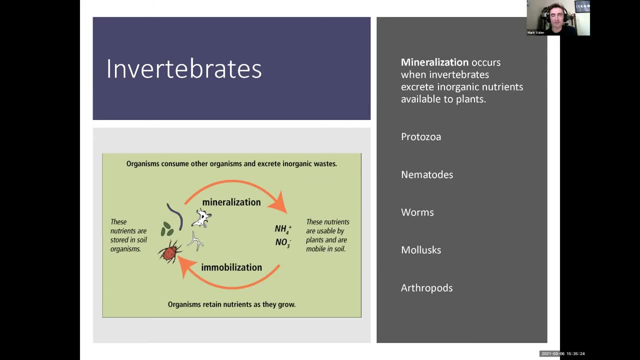 technical, maybe a little hard to understand, But we have that second trophic level: The organisms, the bacteria and the fungi that are living right on the roots, the rhizosphere And the plants we know are feeding those organisms. 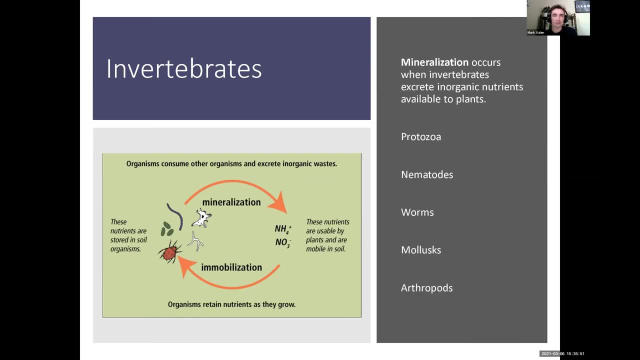 Now, as those organisms take in the sugar and then use it to assimilate the minerals from the soil, it's no use to the plant until that organism somehow releases the minerals to the plant. There's a process involving these microorganisms called mineralization. 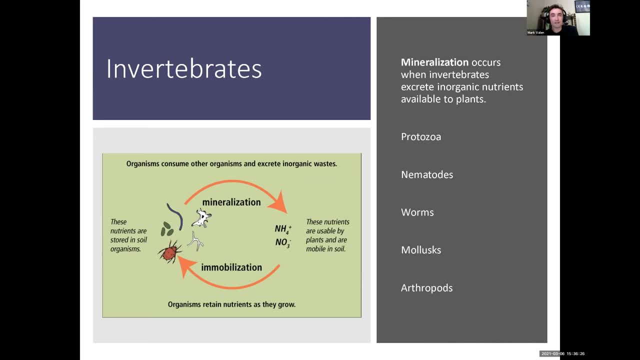 And this involves the living and the dying of the microbes themselves. This is why the third trophic level becomes very important, Because, as organisms consume other organisms, that's the only time that they excrete the inorganic waste products. Because, as the microorganisms grow, 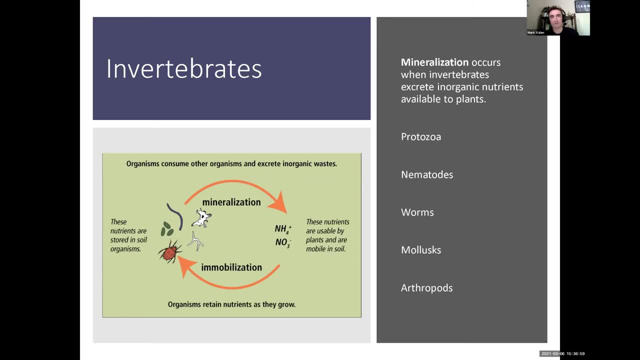 they hang on to these minerals. So that stage of while they're growing and hanging on to them, that's called immobilization, And it's only when the protozoa, the nematodes, the worms, any arthropods or insects 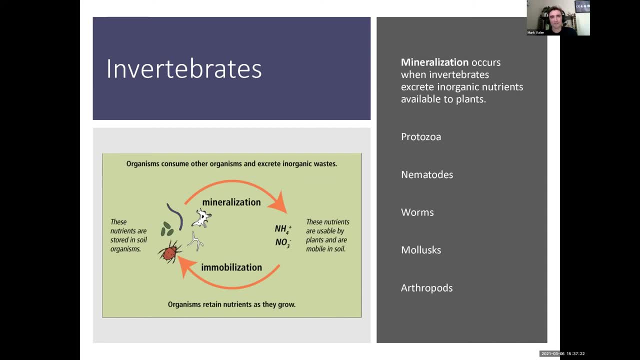 the mollusks, snails and slugs, things like that, when they come along and eat the bacteria and the fungi and then get rid of that as a waste product. that's the first time that the minerals from the soil become water soluble. 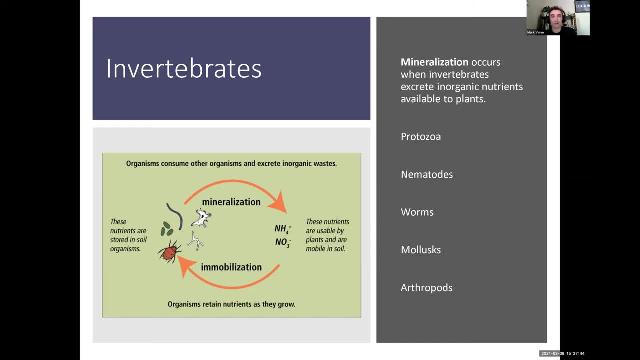 and available to plant roots. So you need all three trophic levels for the soil to truly be healthy. There was a time when horticulturists would look at these microbes and say they're doing a bad thing because they are immobilizing. 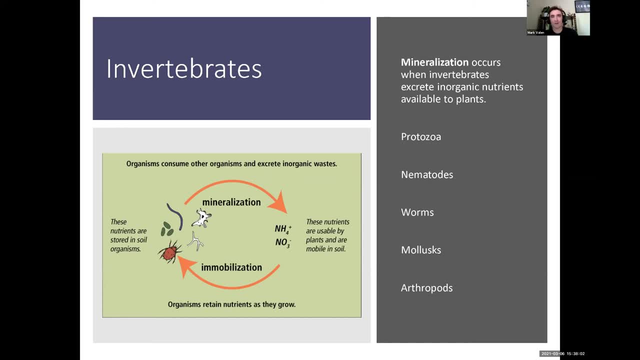 the minerals They are taking up, the minerals that our plant should be getting. So, say, you apply a synthetic fertilizer, which involves minerals that can be dissolved in water. You do not want the microorganisms to drink up all that nitrogen and immobilize it. 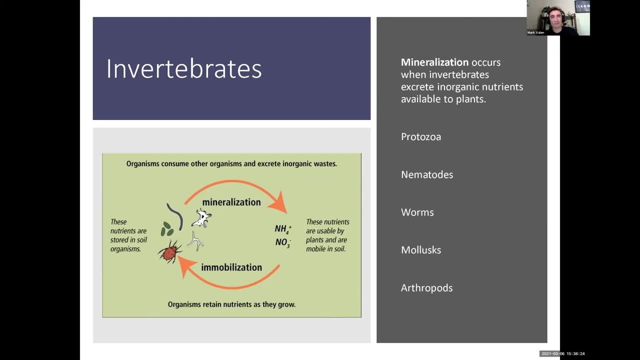 Now, of course, once those microbes die and get eaten by the third trophic level, then later it releases it. But there was a time when horticulturists thought that the soil organisms were kind of opposed to growing plants, And in fact, 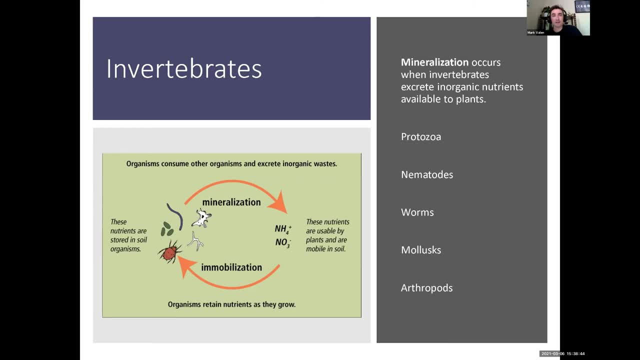 it is true that if you're going to apply synthetic fertilizer, you do want it to go right into the plant as quickly as possible. So it's kind of like you choose one or the other. You choose the synthetic route or you choose the organic route. And they don't really work together very well. If you go synthetic, it kind of pays for you to stay synthetic and be very precise and only apply exactly what the plant needs. The downside is that the soil organisms will not be encouraged to grow. 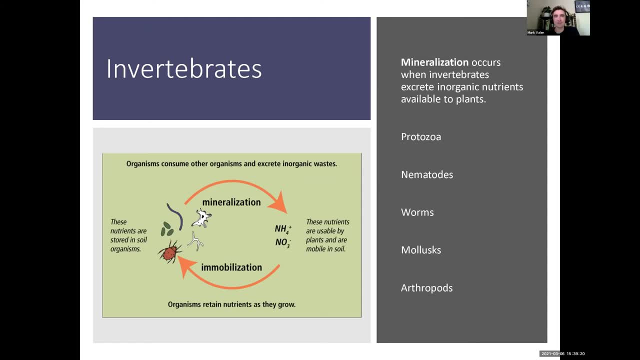 The plant will be so healthy it will not release any sugar down into its rhizosphere, And then you won't have organic matter and all the benefits that it brings. On the alternative side, if you go with the organic route, you should avoid the synthetic fertilizer. 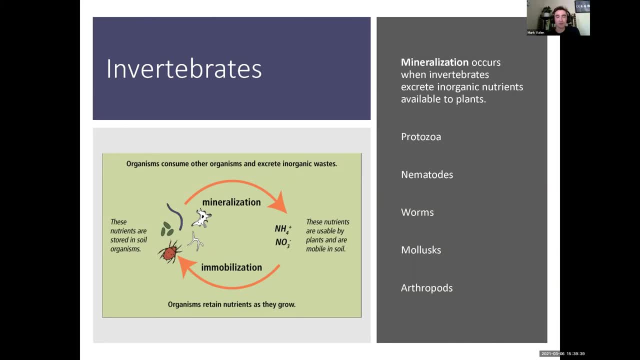 because that can be lost to the microorganisms, It can damage the microorganisms. But the organic route has some downsides too, And it's that it's a little bit of a slower process and it's a little bit less controlled. You don't have the freedom. 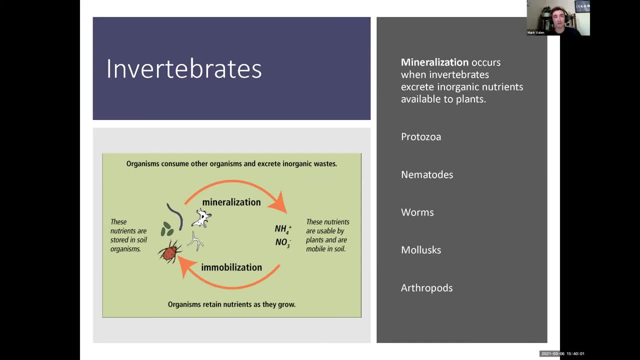 to just put down a little bit of magnesium, for instance, and take care of an immediate deficiency. Instead, you're trying to grow or cultivate an ecosystem in the soil and hope that that will lead to the entire availability of all plant nutrients and some of the other side benefits. 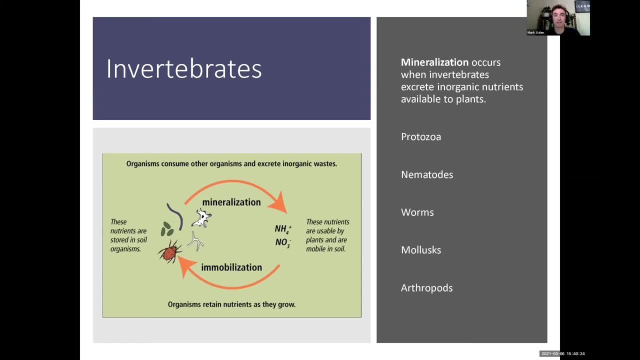 of soil, organic matter, including water retention, proper soil structure and even resistance to plant pests and diseases. So it's not just that you need all these organisms, You need them to be doing their job and you need enough of everything to satisfy, at least. 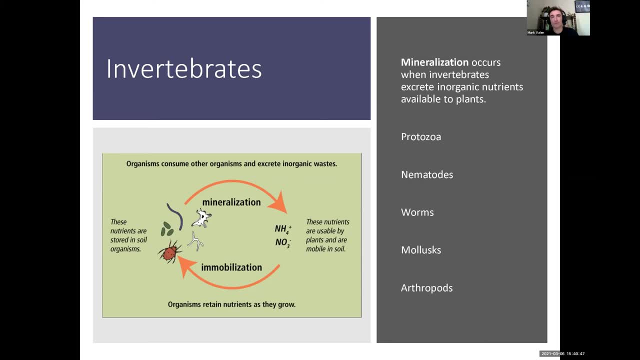 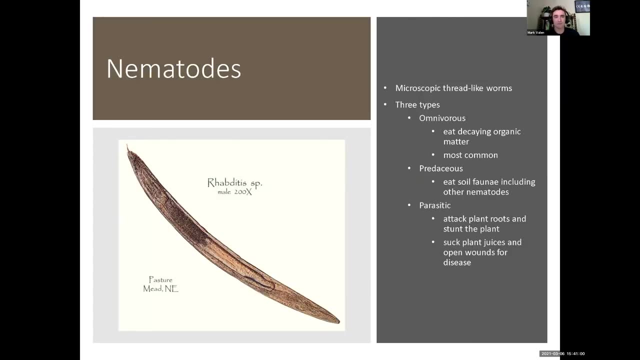 three trophic levels in the soil before any minerals can be unlocked to your plants. So here we have nematodes, And nematodes are just tiny worms, microscopic. So if it's microscopic and it's thread-like and it looks like a worm. 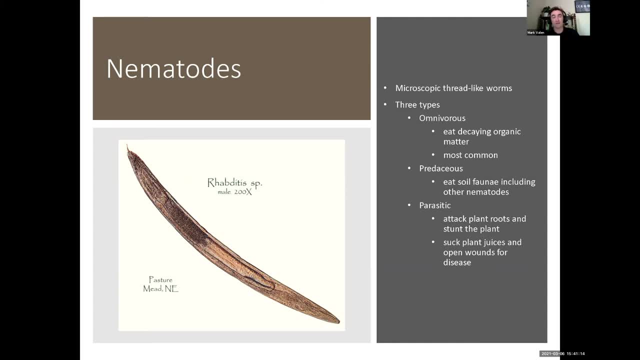 well, that is a nematode. There are many, many types of nematodes. There are omnivorous, and those are the good kind for us, for horticulturists, because those eat decaying organic matter And they're the most common. 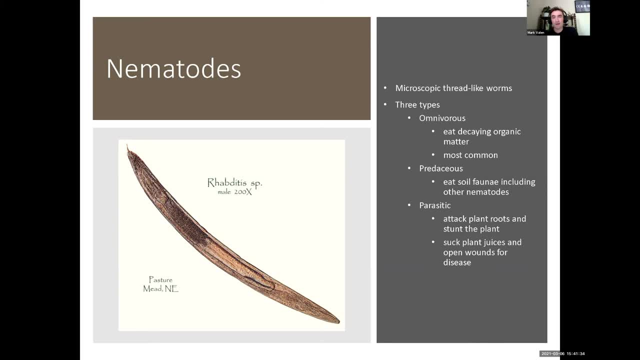 So they're not a problem. Then there are the herbaceous nematodes, And those are the nematodes that will eat other organisms in the soil, And sometimes they'll eat other nematodes too. So these are like the lion nematodes. 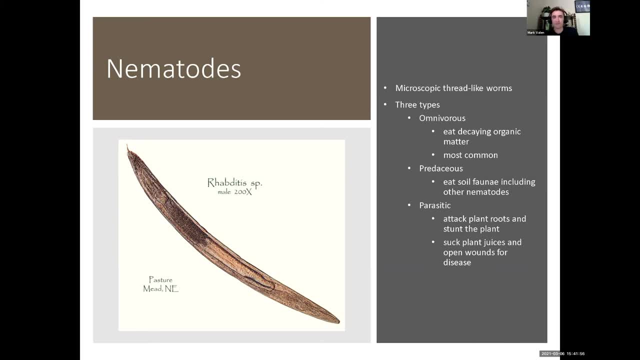 as opposed to the other ones, which are like the gazelle nematodes. And then, finally, we have parasitic nematodes, And these are the ones that horticulturists do not like, because these are the ones that will attack your living plant material. 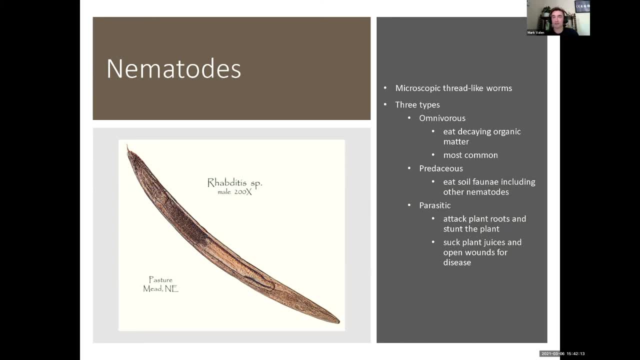 And they're not as common as the rest. So not every nematode by far is a bad one, But the ones that are harmful to plants are parasitic. They will attack the plant roots and it causes stunting of growth And they'll actually suck plant juices. 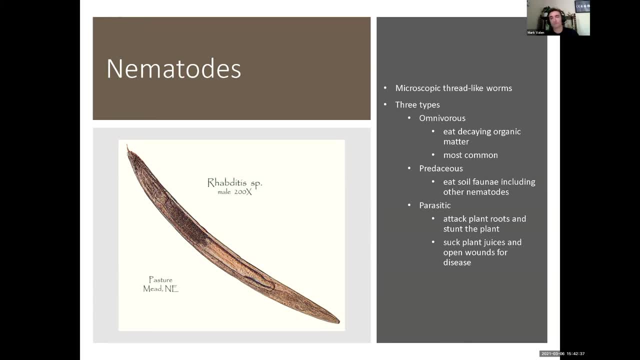 from wounds in the root zone And certain plants will be susceptible to diseases that are brought in by the nematodes. For instance, tomatoes are susceptible to a disease called root knot. They call them the root knot. nematodes Come in and 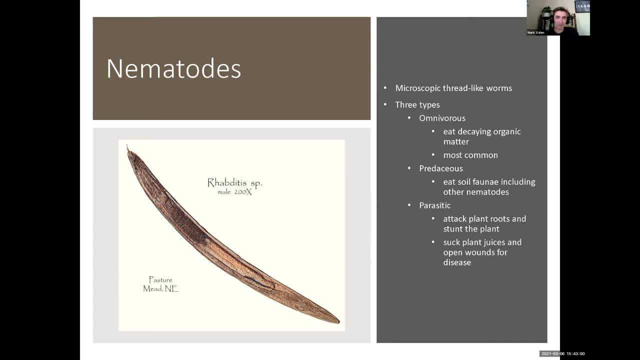 bring the root knot, which actually looks similar to those nodules that you see in legume plants, in beans, But for tomatoes they won't make those nodules. Instead, if you see that and your tomato is stunted and not growing, very well. 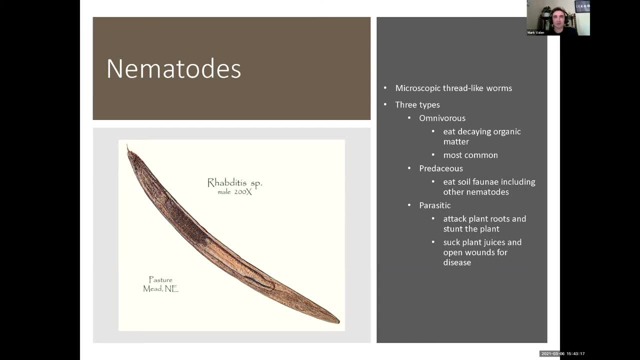 well, you've got the root knot nematode And what do you do? Well, it used to be that you could try to kill the nematodes in your soil, But if you do that, you can kill all the nematodes. 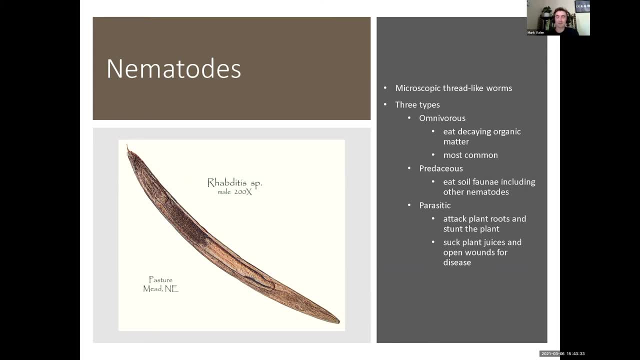 And, as we know, many of them are beneficial, So you can actually introduce predatory nematodes. The problem with this is they're microscopic, so it's hard to know exactly what you're putting and if you're putting it in the right amount. 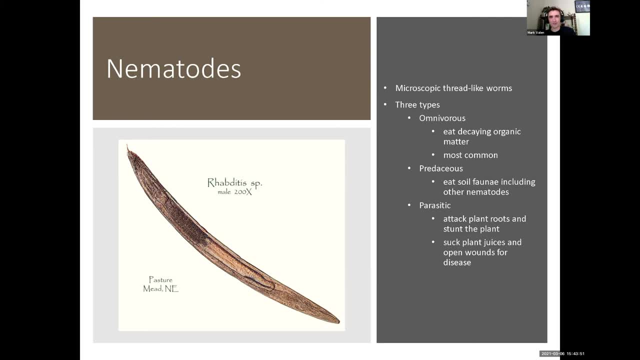 or in the right place. Basically, you go to a nursery, you buy a bag of microscopic things and then you pour out the bag and you hope that there's some nematodes in there and you hope that it solves your problem. 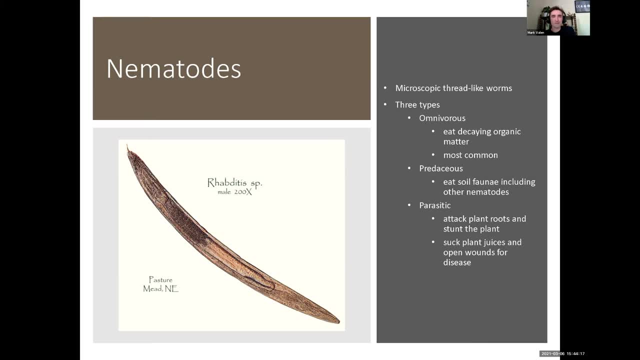 I have a firsthand account of using predatory nematodes and having it work. I'm not sure that it works every single time for every single person. The other thing is, you can try to have a well-balanced ecosystem in your soil And when it comes to gardening. 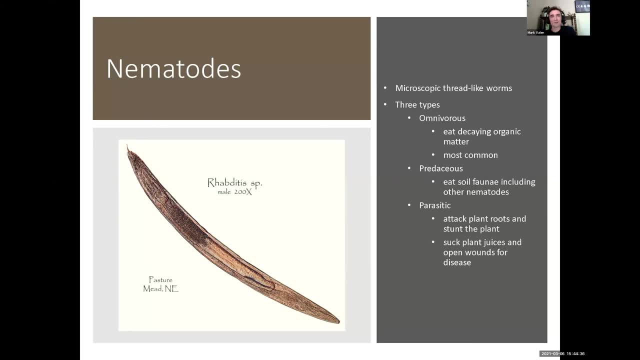 and it comes to tomatoes in particular. this is where some of the traditional practices of interplanting. So you mix some marigolds in with your tomatoes and the marigolds are supposedly either repelling the parasitic nematodes or perhaps they're attracting. 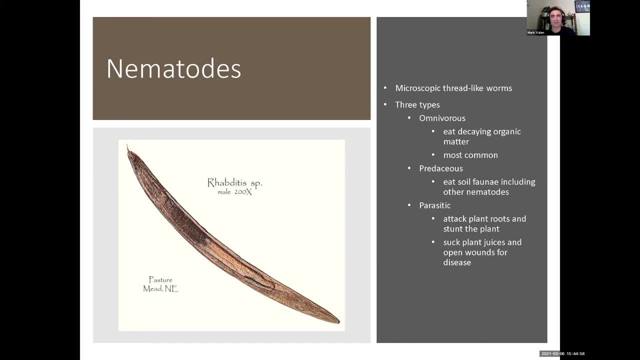 the predatory nematodes. But for whatever reason, if you mix some marigold flowers in with your tomatoes, it helps you to avoid the root-knot nematode. Now, if you get really specialized into the microorganisms in the soil, 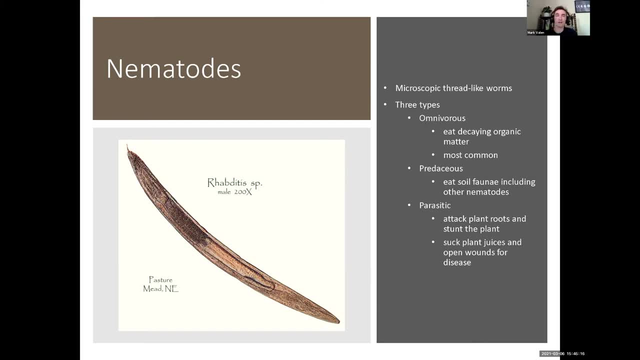 you can look at these under a microscope and they're fairly easy to identify whether it's omnivorous, predacious or parasitic, And the way to do that is to look at the mouth, And the mouth will have different sizes. that indicates basically: 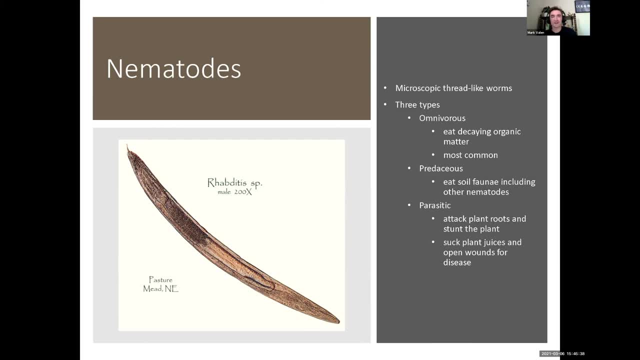 if it has a big mouth it's going to eat larger things, And some of the parasitic nematodes have a spear that's very visible, quite easy to identify, like one single tooth that's sticking out of the front of the little worm's face. 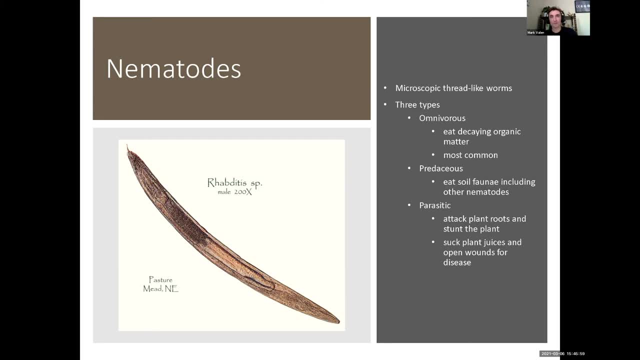 And that spear can actually be thrown and retracted And that's what it uses to pierce into the plant. So if you ever find yourself in the situation where you're identifying nematodes under the microscope, take some time to refer to some reference photos. 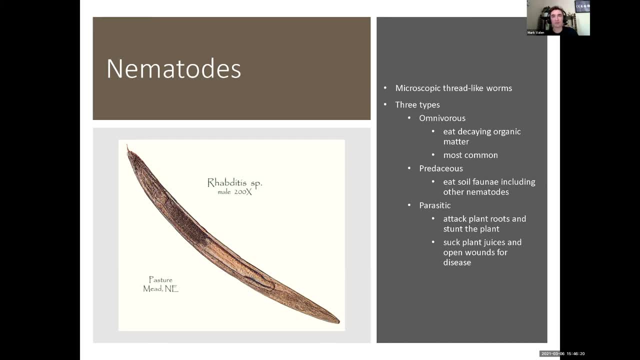 and you're paying attention to the mouth parts in order to see if these are the good kind or the bad kind, And ideally you'll have a balance of everything. And if you have a true balance, then no one individual organism or species can really take over. 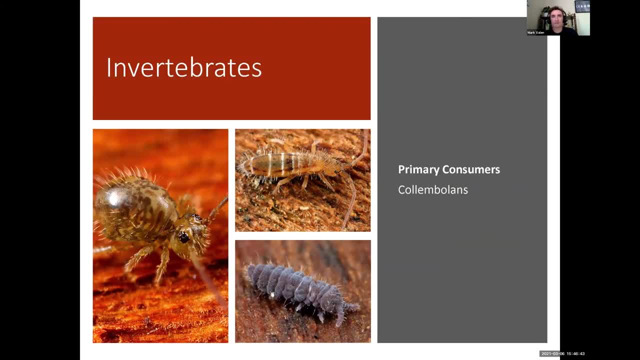 So now let's look at the invertebrates And the invertebrates. a lot of people call them the bugs or the insects. Bugs and insects are actually smaller categories. Scientifically, we accurately refer to these as arthropods, And here I'm just saying invertebrates. 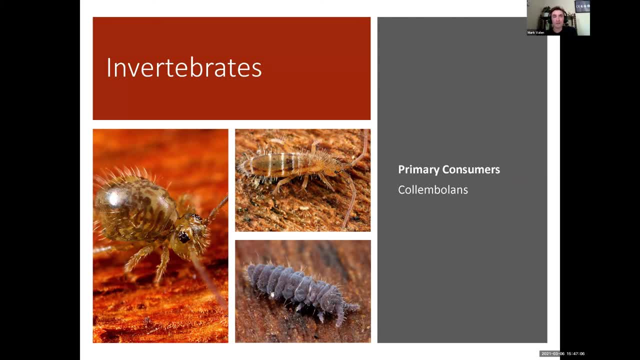 because it's any organism that does not have a spine And typically then it has an exoskeleton. So on the smallest scale of invertebrates, we have columbolins, And they come in all different shapes and sizes for different species. 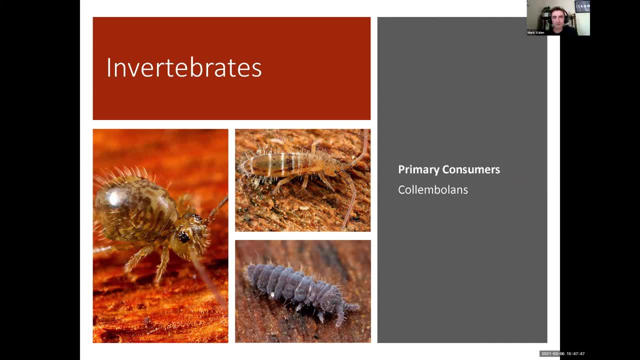 And they can actually be really kind of charismatic if you look at them under a microscope and kind of cute. And you see a few photos here: The one on the left obviously much shorter and rounder, The one on the right more elongated. 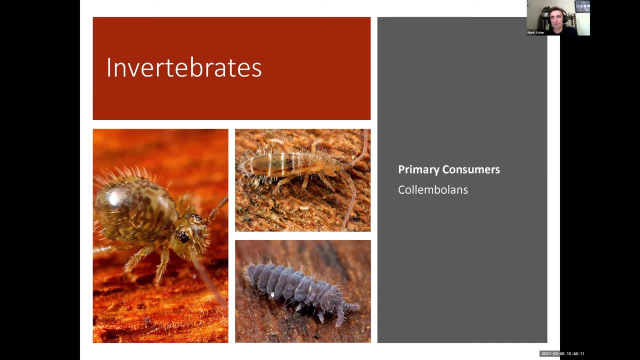 And you can see a larva of one down there as well. Columbolins: These are called primary consumers And therefore in the soil they're considered to be the second trophic level, because they are eating the decomposing organic matter. 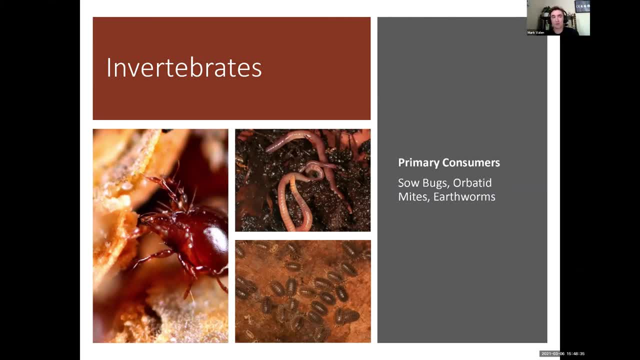 Still in this same category of primary consumers, but going up in size. these are things that are easy to see with your eye, And the smallest thing you can see with your eye is pretty much the orbaded mite. That's the image on the left-hand side. 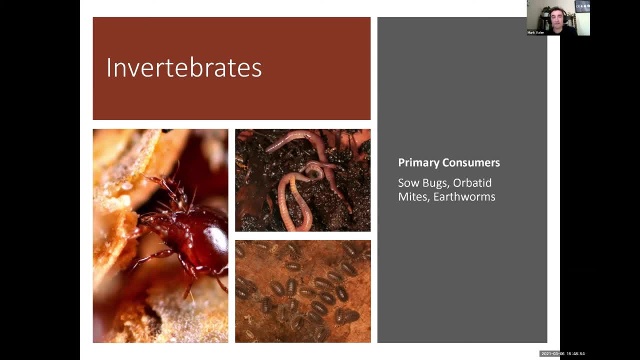 So a mite is related to a spider, It has eight legs And the orbaded mite is about the size of a period if you're writing with a pen or a pencil. So the tiniest little dot you can make. 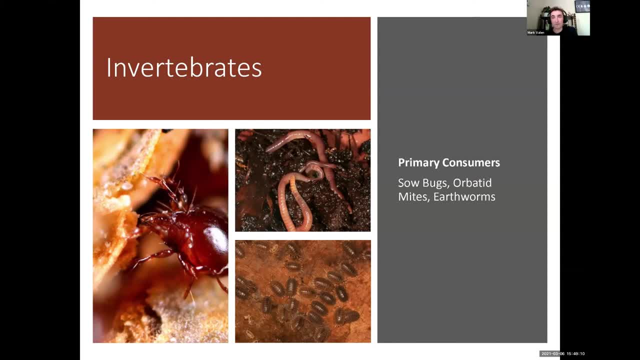 that is an orbaded mite And they're very round, So they have the orb shape And typically red or black in color, So somewhere kind of a dark red or a black color, And you can see them moving around on decomposing organic matter. 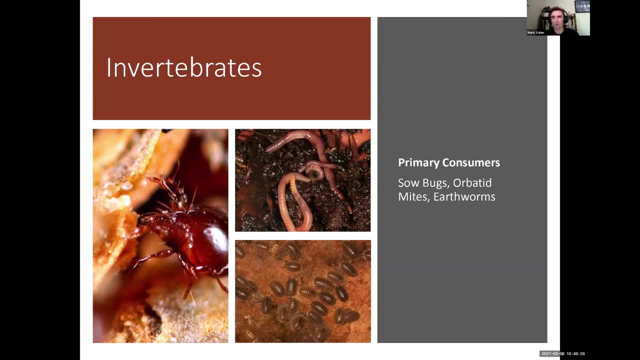 especially in compost piles and worm bins and things like that, But they're out in nature in our soils as well. We have sow bugs, which are what most kids call roly polies, And there's kind of two main types of them. 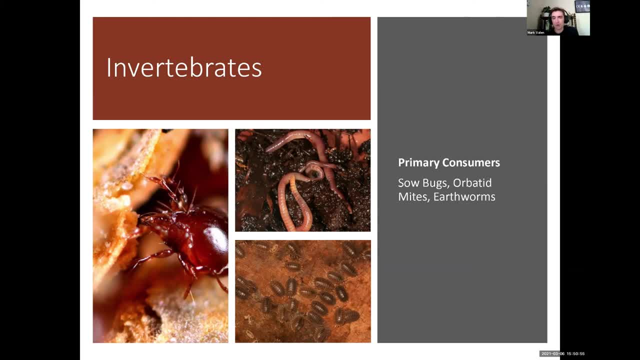 There's the sow bug, which is a little bit more flat, And then there's the pill bug, which is a bit more rounded, And the pill bug is the one that can actually fully roll up into a circle. Both of these are commonly referred to. 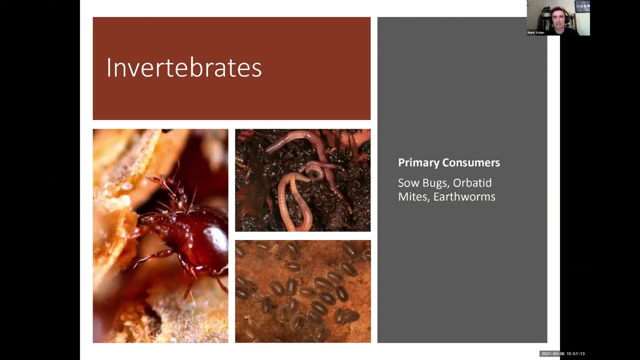 as wood lice, Wood lice. It moves around and feeds on all of these plants and clients. But the pill bug has sort of a general name And technically they are crustaceans very similar to a lot of aquatic organisms And not truly native to our area. 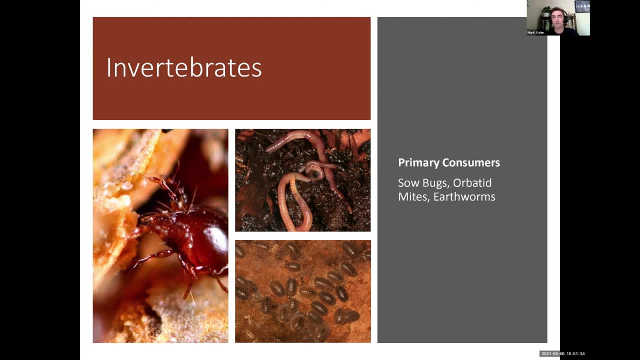 So there's not a lot of things that eat them. In fact, these can be primary consumers of dead plants, but also these will eat living plants. So too many sow bugs, And then, of course, we have earthworms. There's many species of earthworms, and they do a fantastic job of decomposing plant material. 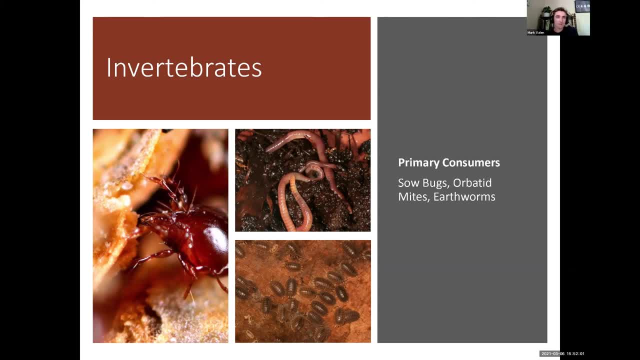 They don't have any teeth, but they have a special combination of microorganisms inside their digestive system, So as they pull food in, it combines with all the different microbes inside of their bodies and they actually release the food back out in both directions. 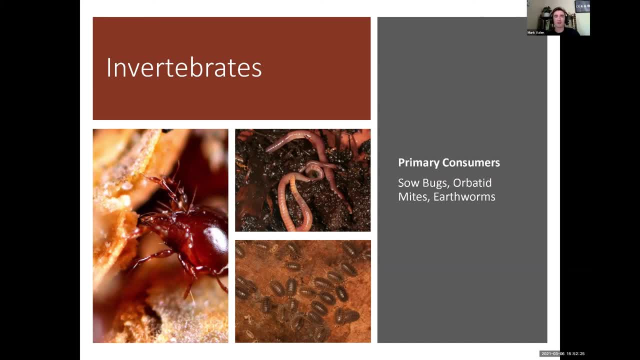 Sometimes they spit it back out and they'll eat it again. and then other times it comes out the other side and they'll eat it again. And it's just this little ecosystem where the worm is constantly cycling The old, The old, decomposing plant material and every time it does it infuses that product with a high-quality dose of a wide variety of bacteria and fungi. 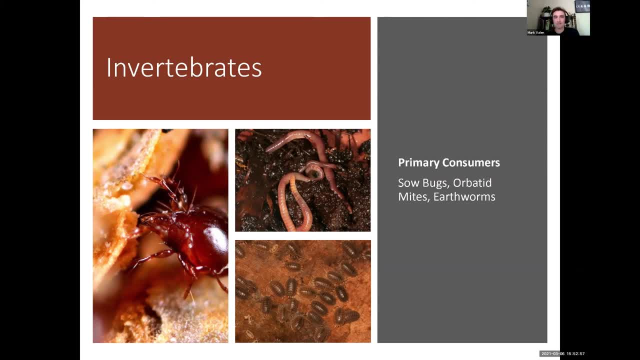 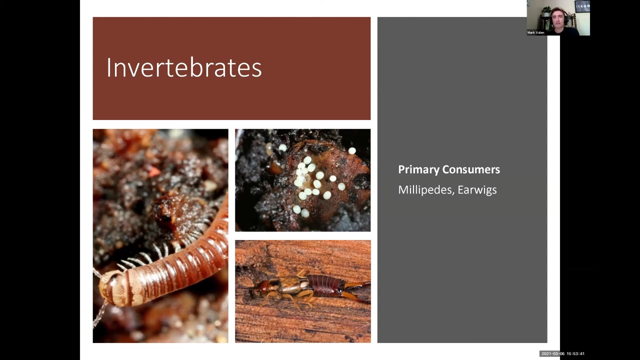 That's part of the reason the worm castings, the byproduct of the worms, is so rich in plant nutrients and why your plants respond so quickly. It's because it's charged With beneficial microbes. In natural ecosystems as well as in the garden. we have millipedes and we have earwigs that we commonly see living in and on top of the soil. 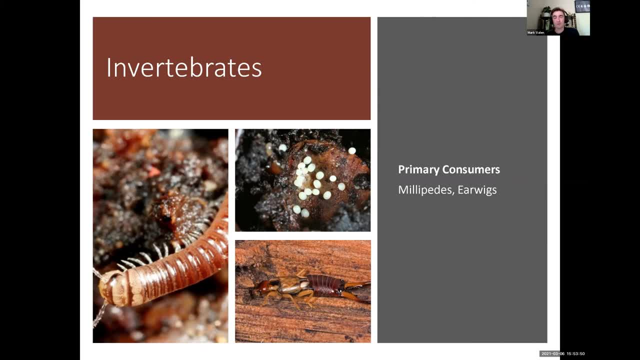 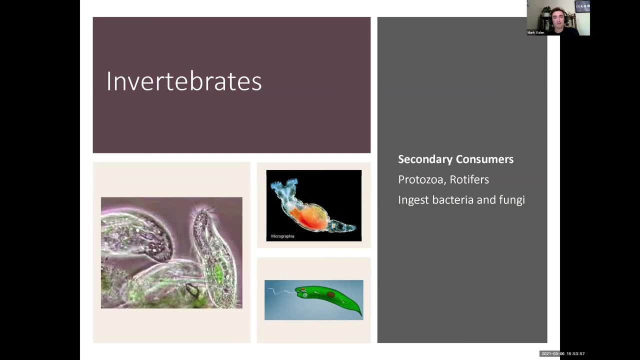 And again, these are still primary consumers, even though they can be quite large and easy to see. And now let's take a look at secondary consumers. So these are the third trophic level. These will not be eating organic matter in the form of dead, decaying plants. 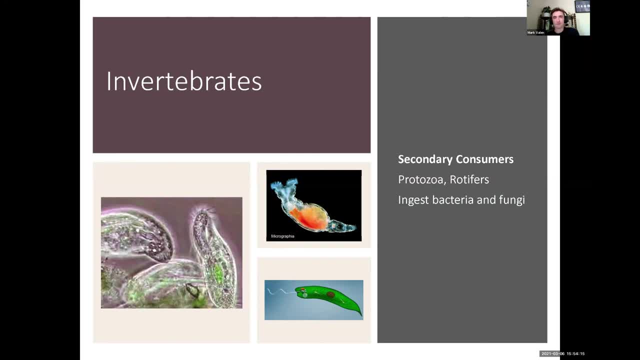 These are going to eat the bacteria and the fungi that eat your dead, decaying plants. So these are secondary consumers And we have protozoa, which is what we're seeing on the left-hand image. On the left-hand image That looks to be a ciliate, so you can see all those little hairs on one end and those are called cilia, and so if it has all those hairs, we call it a ciliate. and then we have a little moving diagram on the bottom of a flagellate. a flagella is a single longer tail or hair that can move to help propel the organism. 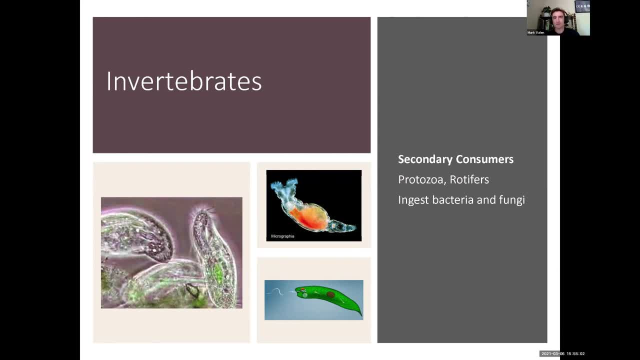 So we have a flagellate, which is a single longer tail or hair that can move to help propel the organism. So we have ciliates, we have flagellates, and then we have a rotifer, and that's the image on the top right. 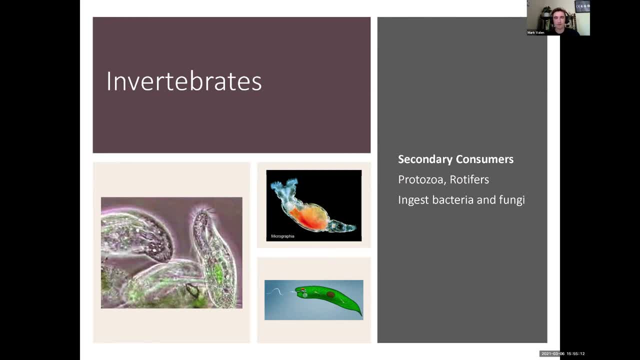 And you can see the head and the tail of the rotifer. and the head has two sides to it, two jaws and little cilia are on both ends and those will move in coordination so that it actually looks like a little conveyor belt. 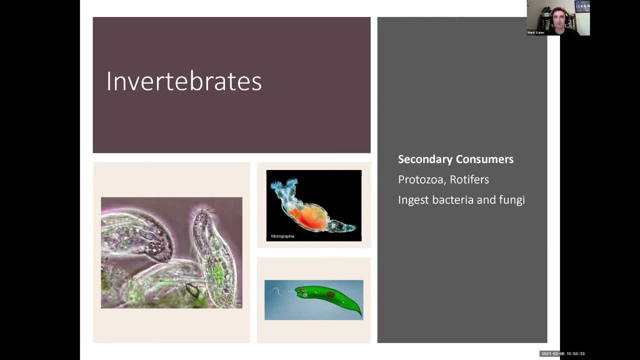 That's, That's That's That's That's Rotating, which is where it gets the name rotifer. But these are microscopic, you cannot see these with your eye and these live in water. So these are aquatic organisms and remember, the soil has water all the time. 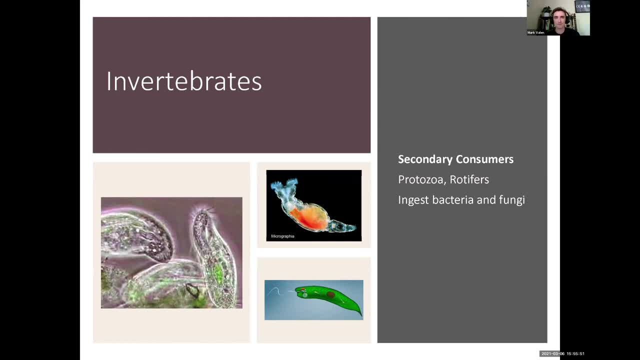 And in that water these organisms live And these are the predators. so they don't need to be large, they can be small. But if you have these types of organisms in your soil, then you know you are having mineralization, You are having 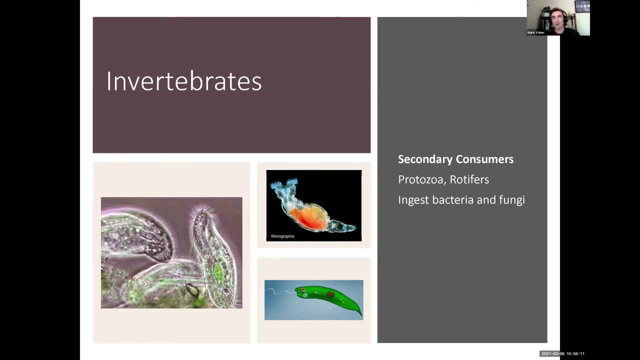 the immobilized minerals that are trapped in the bacteria and fungi. You're having them released once they're consumed by these secondary consumers and becoming available to your plants. So these are the good guys. If you ever look in a microscope and you see these, that's a great sign. 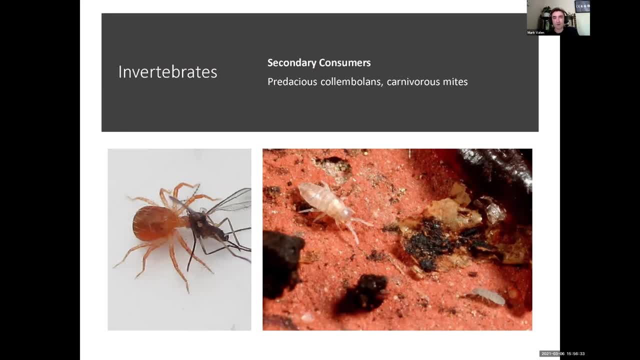 And now for our larger decomposers. we have larger predators And so we have predatory columbulans. The image on the right you can see a large columbulan going after a small columbulan, And the large columbulan is the predator, The small columbulan is the decomposer. 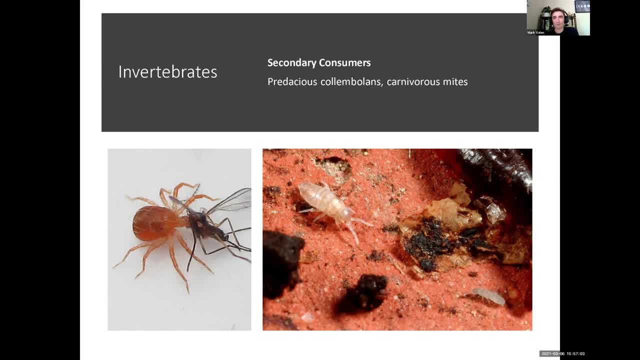 And so you have a whole world taking place down in the organic matter layer of the soil. We talked about the orbated mites as being primary consumers. Well, the image on the left-hand side is showing a carnivorous mite. Notice it has eight legs, So it sort of looks like a spider. 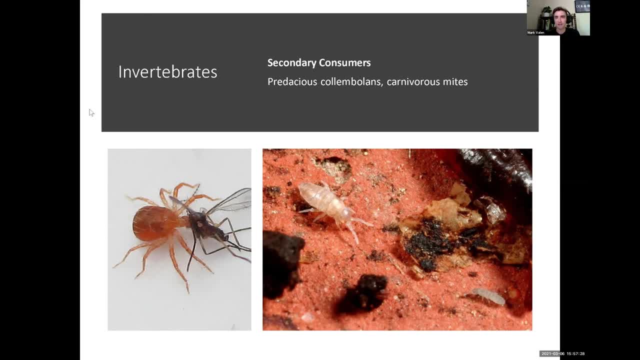 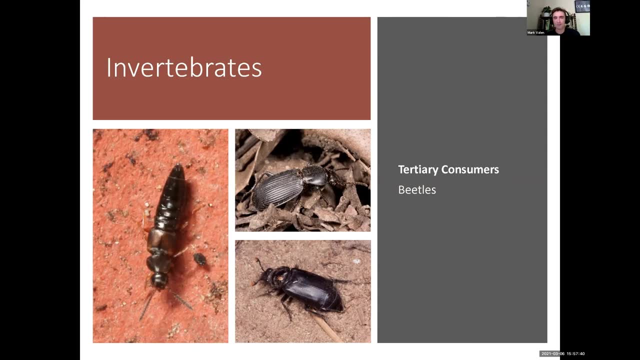 And here you see the image of it going after a little fly or a midge, And then we get up to tertiary consumers. These are the larger creatures in the soil that will eat the secondary consumers, or the things that will eat the predators, And primarily these are beetles. So you start getting into the larger organisms. 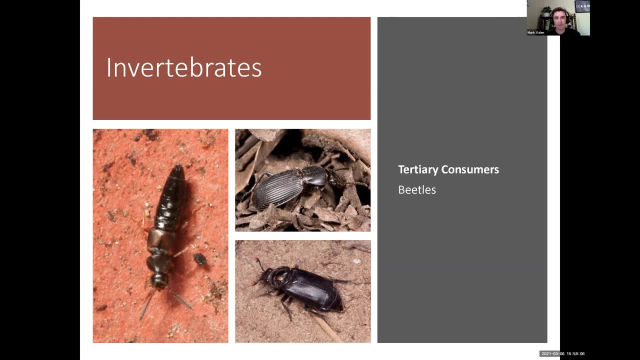 And many different types of beetles exist. One thing you can note on the, The image on the bottom right: that beetle. do you see that it has its own parasite? So it has. There's a mite that is riding on the beetle. So, even though the beetle is a 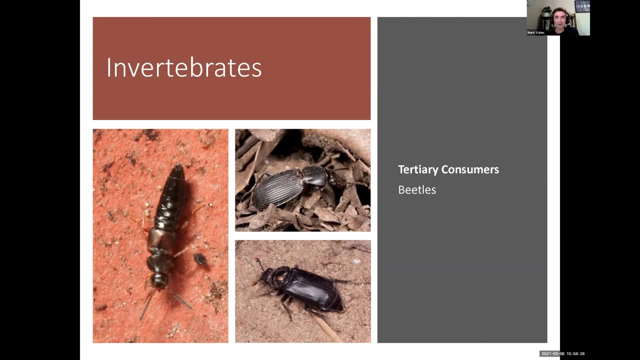 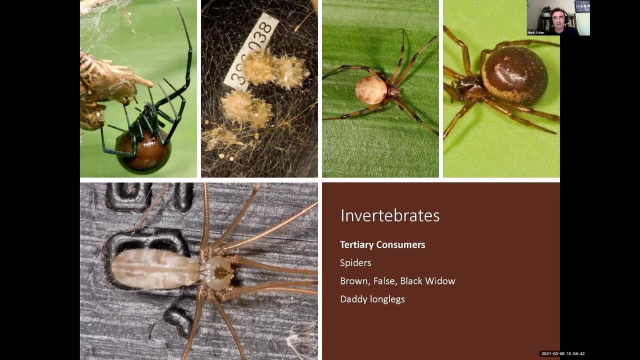 top predator in the soil, there are other organisms that will still feed on the beetle as a parasite, And so everything. The web gets thicker and thicker the more connections there are, And so it is mainly двухлагgedちゃ. In addition to other species of bugs, they can also take害. Do not fear if you have a spider. Spider means you have a healthy ecosystem, And so, therefore, you have to have a lot of all those nice, airy and Reiw greater cercid. species, all in one тысяч very good messed up umpires. So just pictures to let you know they are toys there and there. For some of you this is the lにちは house. But one fact we would find so interesting: axle and map wanting to walk the halls of Dorset. so water. I basically agree with Matt when he talks and try not to just grammatically describe them. You see how places have sort of crossed across them in the characteristics. What do you mean? It's all. Wherever did I say all of these places? from style, though. 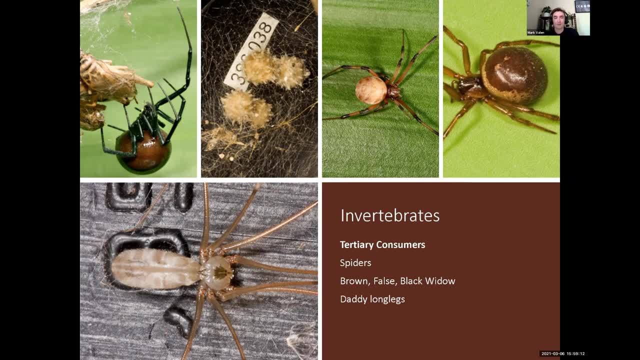 I'd be right. This is unusual if it was just a label of all the trophic levels below So many different types of spiders. they're all predators, they're all good. Do not worry about avoiding any kind of spider from a garden perspective. 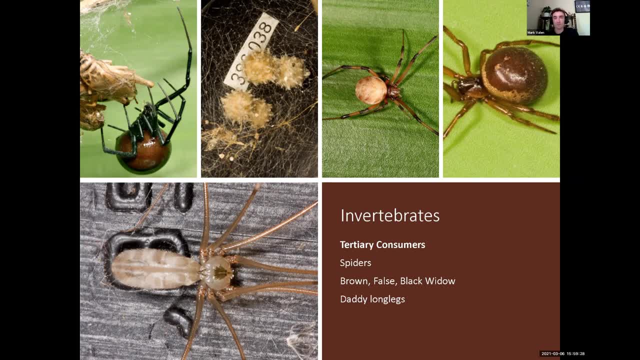 Now, of course, some spiders can give people a bite. black widow, brown widow- A lot of people say the brown recluse, although we do not have them in San Diego, even though the doctors will sometimes prescribe or diagnose a fungal infection of your skin. 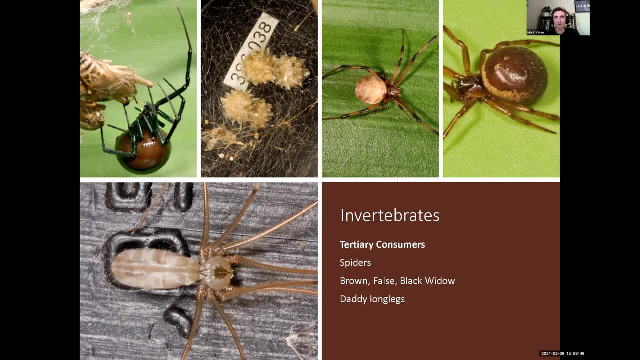 as a brown recluse. There are no records of brown recluse in San Diego. If you find one, you can turn it into the Natural History Museum and they'll pay you $1,000 if it's really a brown recluse. 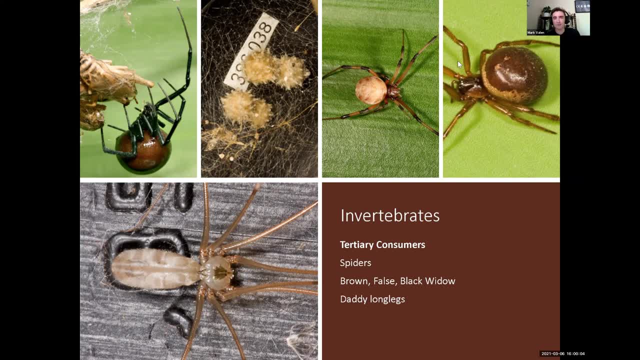 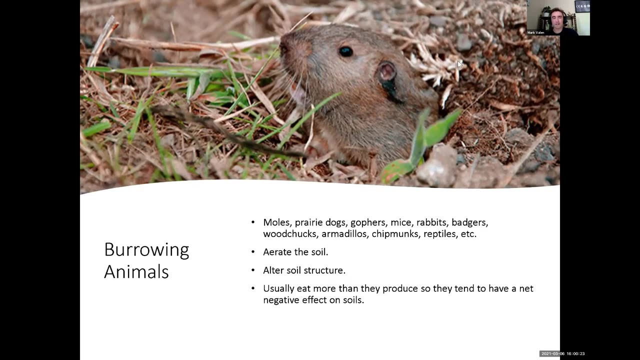 because there's a lot of misinformation out there and we need to help people understand what's really going on. So don't go killing spiders trying to get $1,000.. The thing is, you're not gonna find one. And then, finally, if we get to the even larger size, 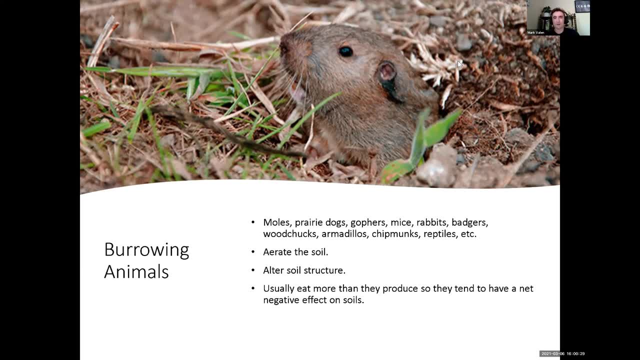 we have our animals, which are all sorts of different categories of animals, but we tend to think of the mammals. So here's an image of a gopher, a pocket gopher. And again, traditionally horticulturists don't like the gophers. 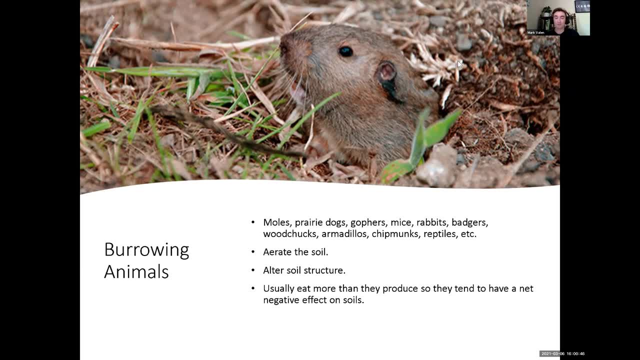 because they don't like the gopher, Because they will eat living plants- and it's true, They will eat living plants. And it's problematic for your plants because, in particular your trees, your young trees, the gopher can eat a lot of the roots. 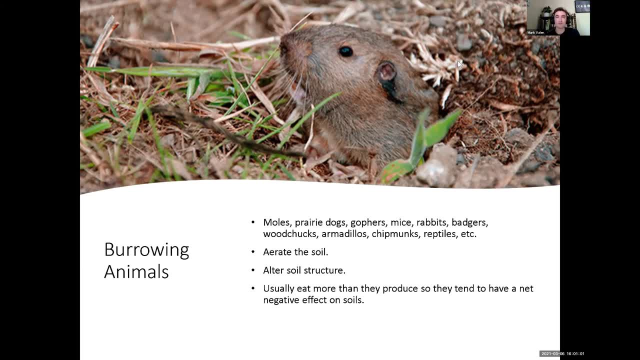 before you even know that the tree is suffering. And then one day the tree just falls over and dies and you look and you discover that gophers had been eating the roots for a long time, And in a natural eco-system though. 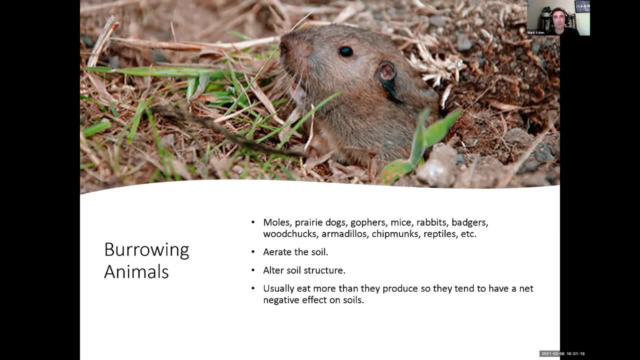 that's a small price to pay for the benefit that the burrowing animal does. So there's. you can imagine the aeration and the change in soil structure that takes place when you have all of these types of animals: moles, prairie dogs, gophers. 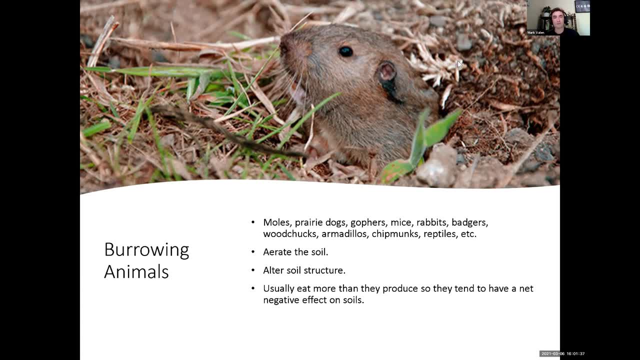 even mice and rabbits and all the animals that dig burrows. that has an impact on the soil in a positive way, So it aerates the soil, It alters the soil structure And in a garden setting, however, you want to try to be smarter than nature. 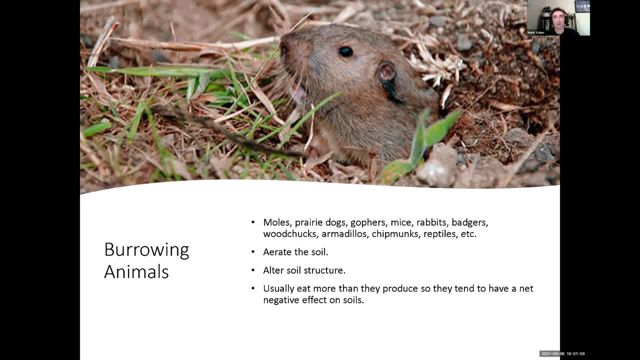 You can't blame the gopher for acting like a gopher, But if we learn how the gopher lives, we can try to design a system that does not favor the gopher in our yard or in our landscape, And so there are techniques to try to discourage gophers. 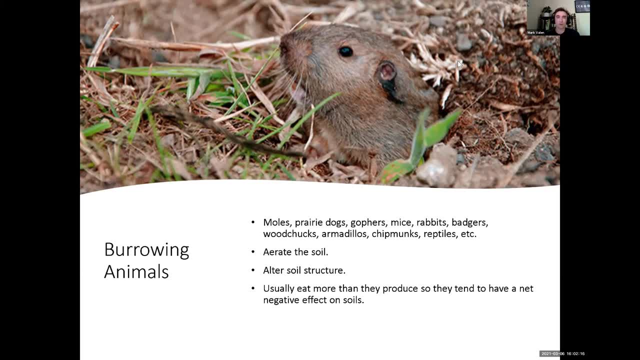 one of those would be to plant bulbs like daffodils right in the same place as your trees, because the gopher is said to not like the taste of the daffodil, So if there's daffodil close by. 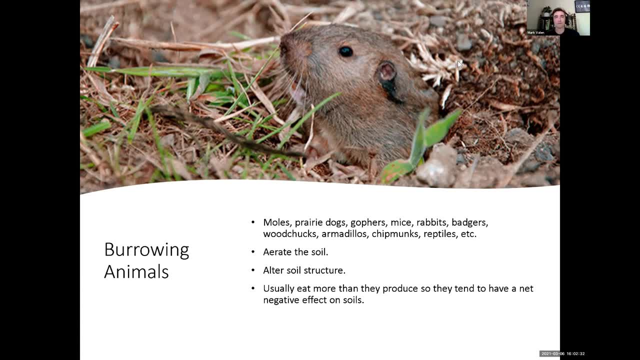 the gopher will go somewhere else. And the other thing you can do is have a cat around, because the cat, first of all, a cat will chase a gopher, but second of all, just the smell of the cat in the yard. 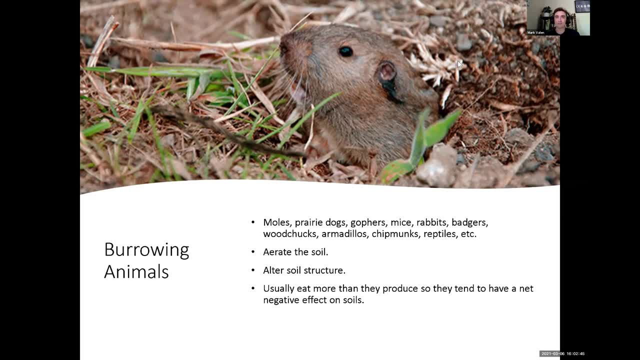 will be a problem. The landscape will discourage the gopher from being there And, of course, if you need to on a farm setting or if there's any kind of true problem, it is legal to trap and control for the gophers. 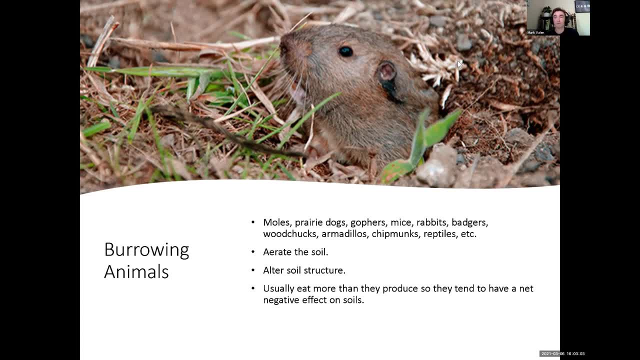 But we always want to do that as a last resort because we recognize that they have a valuable impact on not just the soil, the soil structure, but now that we're getting into larger animals that's going to be part of the larger ecosystem outside of the soil. 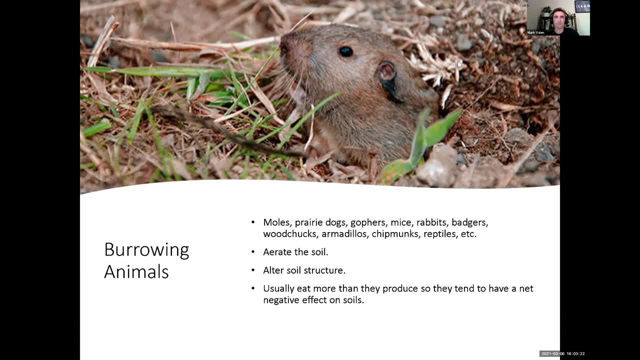 So we have our coyotes and our birds and all of the intricate connections of nature being involved, And so these larger animals, traditionally in horticulture, were just seen as a problem. Kill them or get rid of them, And the fewer organisms the better. 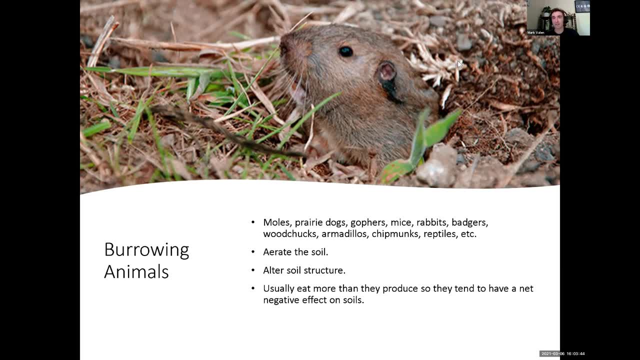 because all the animals are just competition for our plants. But now we recognize that if we work with nature and try to go with the direction of ecology and relationships and understand them better, then we can have nature do a lot of valuable services for us. 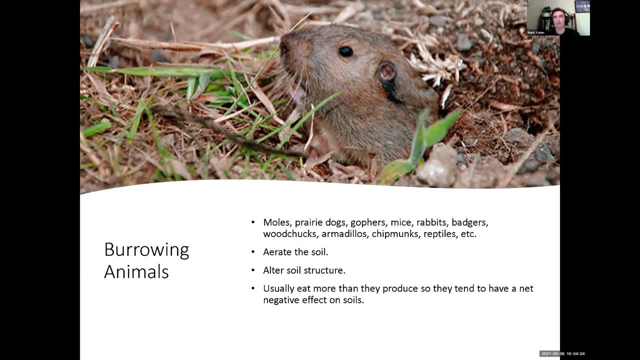 And our plants can be even healthier with less input from us: Less work, less time, less maintenance, less energy. But the problem is we have to be smart and we have to understand how it works, and we have to put it all together so that the puzzle pieces fit naturally. 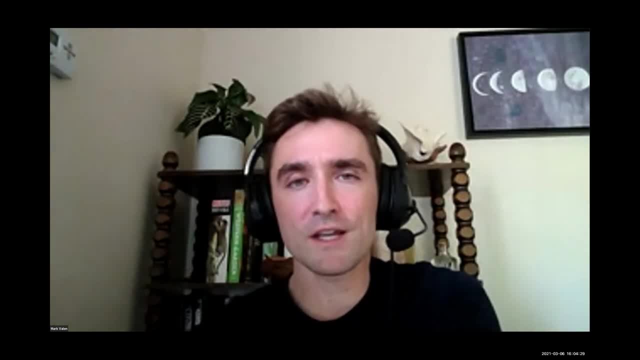 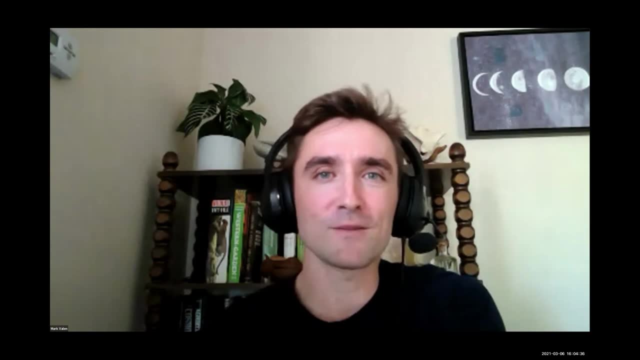 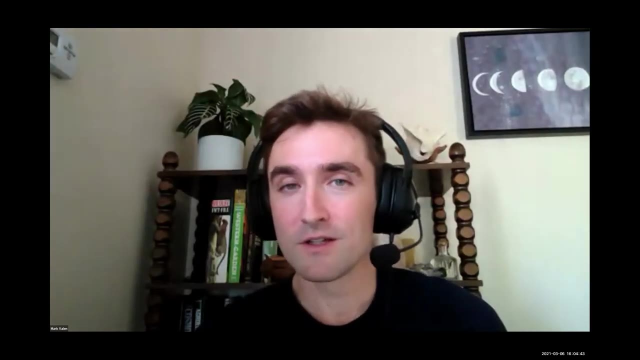 So there you go. That's an introduction to soil ecology and the players, all the components, the living components of an ecosystem. And remember, the ecosystem is the study of the organisms and how they relate to each other. So keep in mind those.